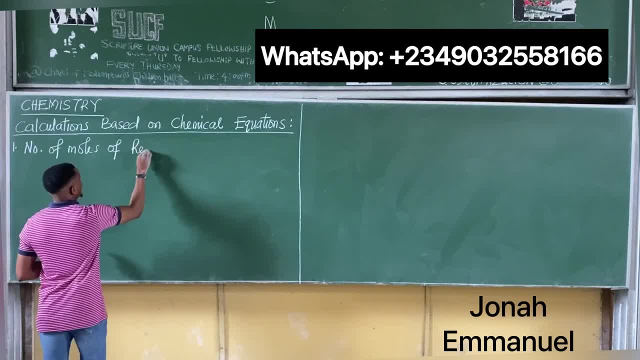 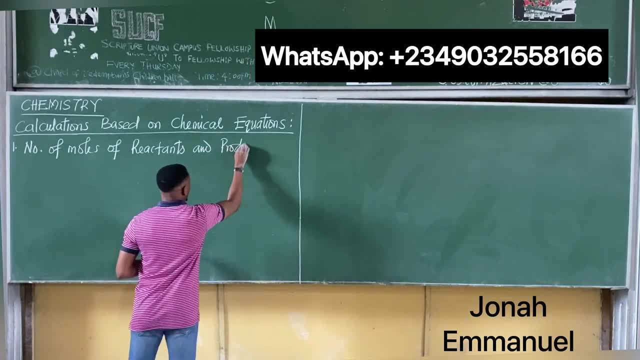 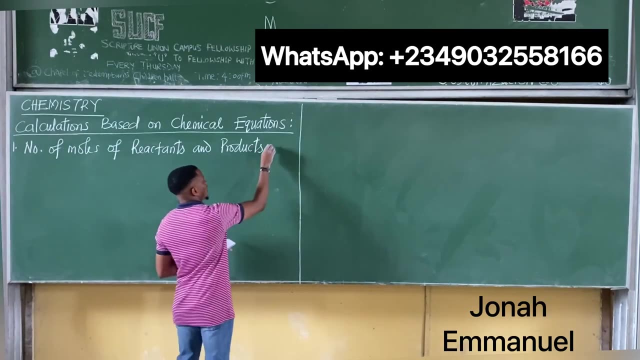 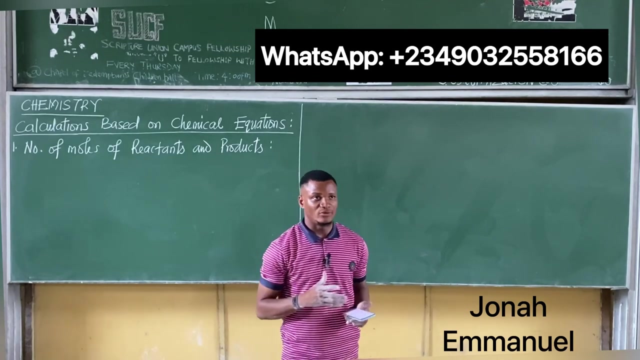 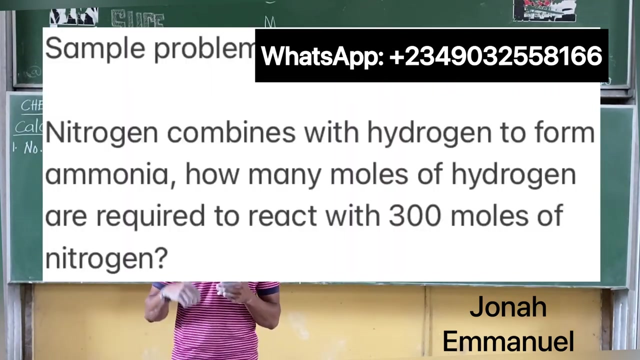 of reactants and products, please. So what kind of calculation we can do on chemical equations is the number of moles of reactants or products? I'll take a simple example, I'll explain this and we proceed, please. Example example: nitrogen combines. 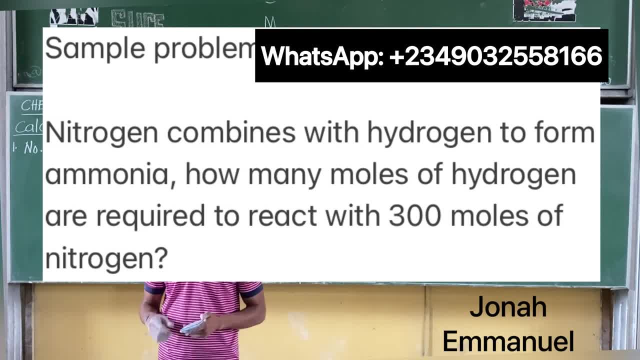 with hydrogen to form ammonia. Nitrogen combines with hydrogen to form ammonia. How many moles of hydrogen, How many moles of hydrogen are required to react with 300 mol of nitrogen Are required to react with 300 moles of nitrogen. How? 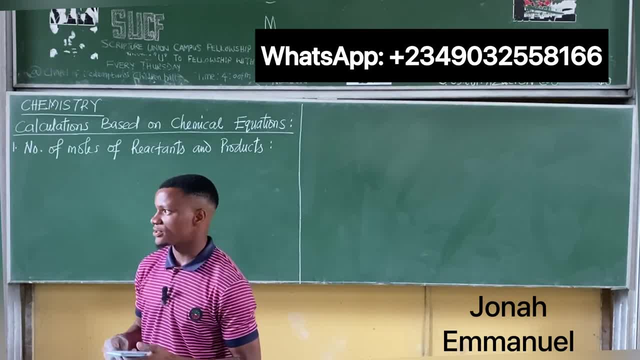 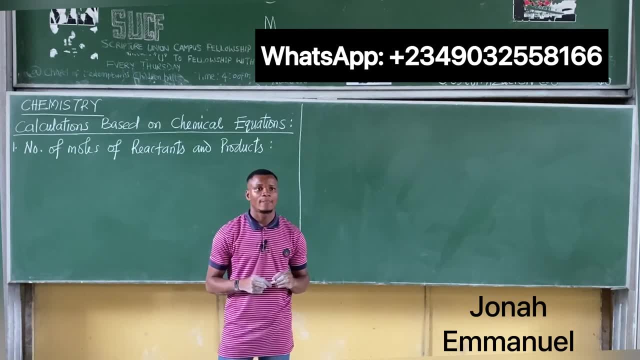 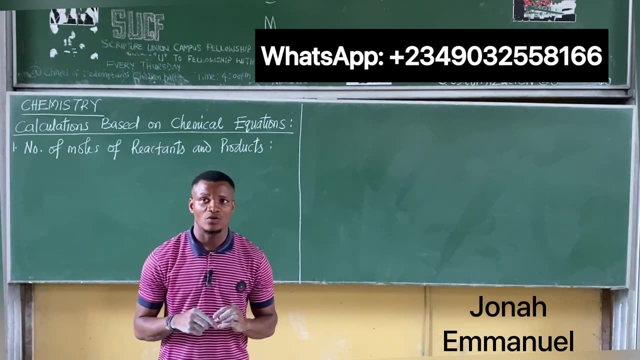 many moles of hydrogen are required to react with 300 moles of nitrogen? officer, lol, For questions of this manner, Science also käyt. your first task is to write a balanced chemical equation in your test, which we'll do shortly. you observe that- to first of all give you 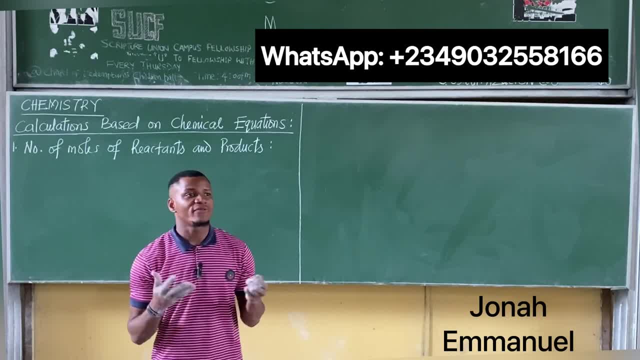 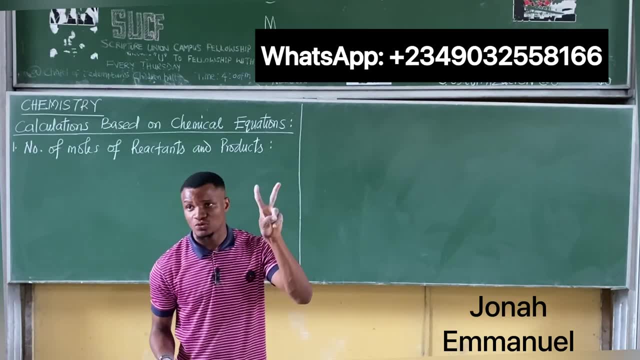 the equation, but then let's assume we're not giving the equation. so if I look at this head, nitrogen combines with hydrogen to form ammonia. my reactants are two nitrogen hydrogen, my product is one, ammonia. so okay, on your own. 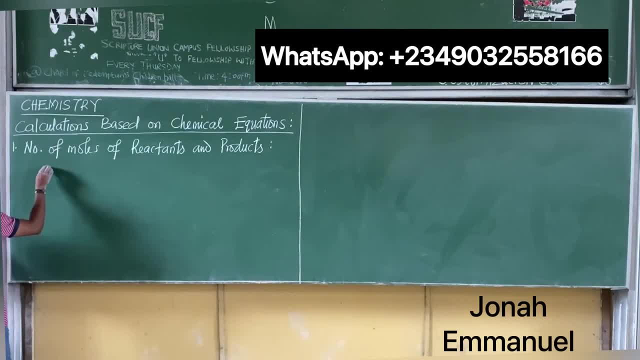 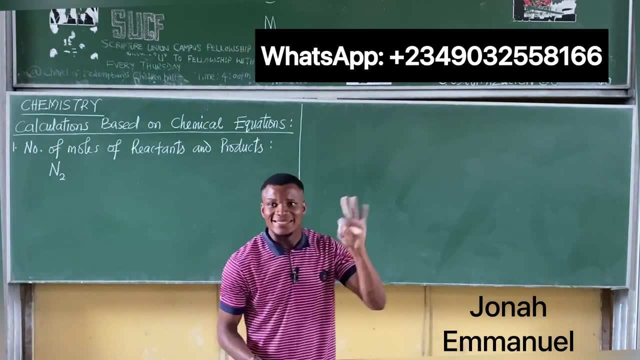 please, but let me save time. this I'm recording: nitrogen is what there, not N, N2, now this is where people will miss it up at this point. now note the atomicity: nitrogen is not N, it's what there, N2, it's diatomic. 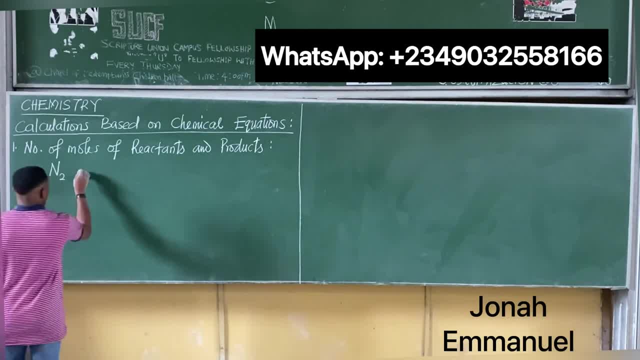 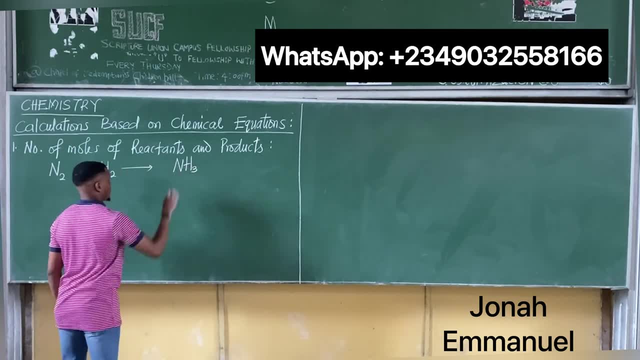 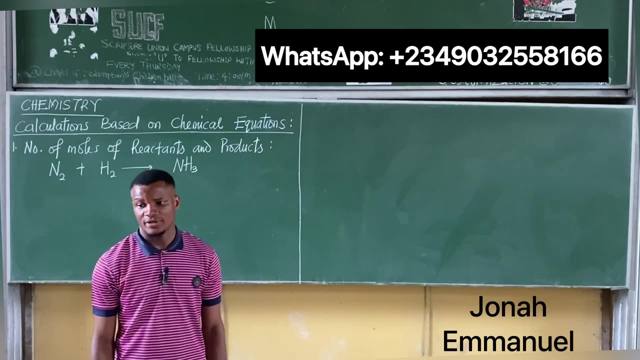 plus hydrogen H2, to give you the set ammonia. ammonia is NH3, please note. so, please note, nitrogen is diatomic. it's not N, it's N2, it's diatomic. so I'm having this one here, so I'm having nitrogen. 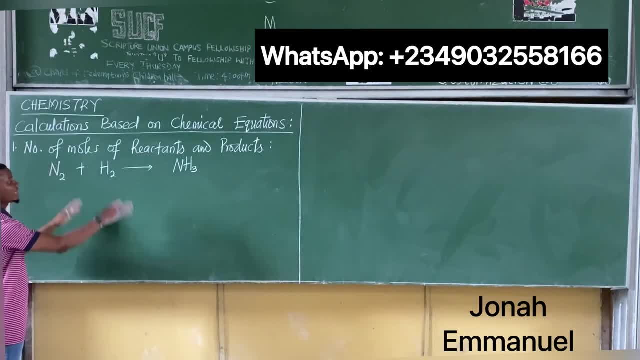 combining with hydrogen to form ammonia. we said we cannot work on this except first of all we balance this. in balancing this, I'm seeing 2 of nitrogen. this is 1, I'll simply add 2. here we add whole number coefficients, of course, 2 times. 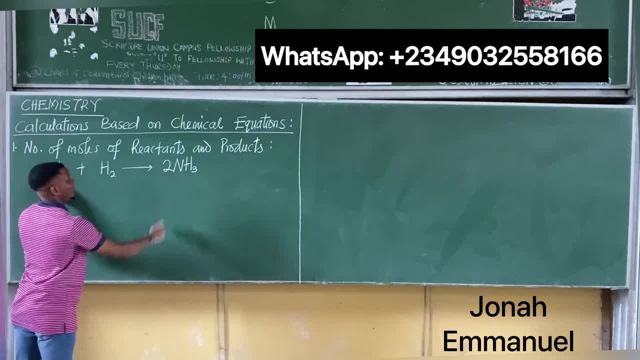 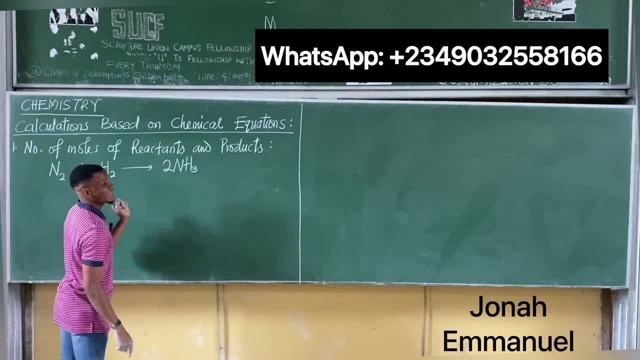 1 is 2, 2 nitrogen here. 2, here is balance hydrogen. I have just 2 here, for here I have 2 times 3, that's 6 hydrogen. 6 here, 2, here I'll simply add what there, 3, so it becomes: 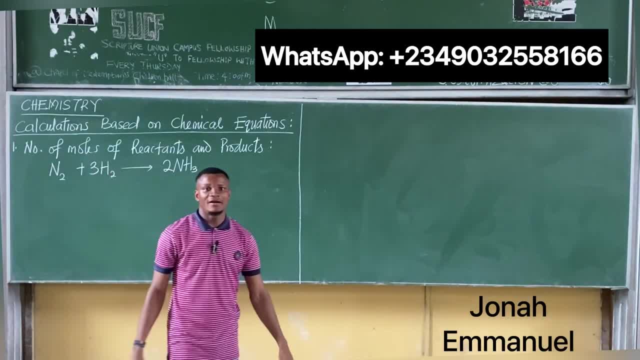 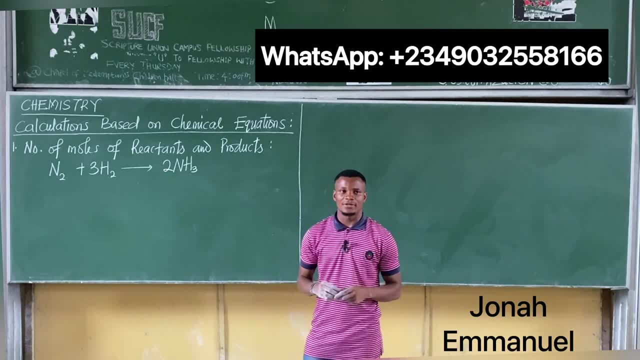 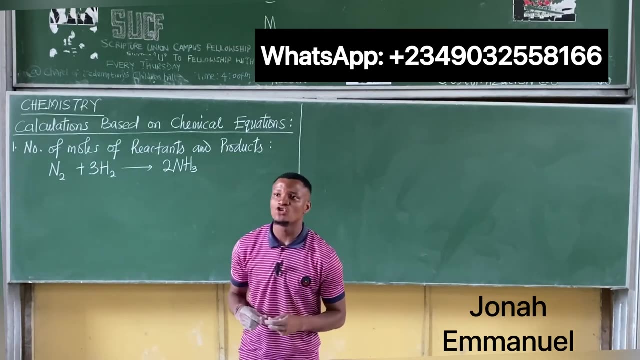 3 of hydrogen at this point. now I have a balanced chemical equation. my first task when it comes to balancing chemical equation. what's next? the next task is to get what is called molar ratio. what's molar ratio? molar ratio is simply the ratio of the coefficient of each of the reactants and products. that's all. in other words, for this case, molar ratio. molar ratio becomes coefficients. here is 1, ratio is 2, coefficients here. 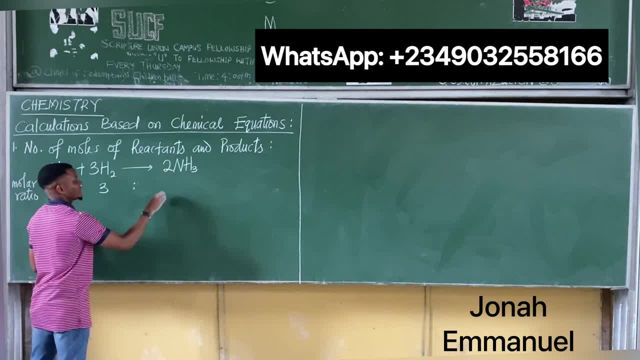 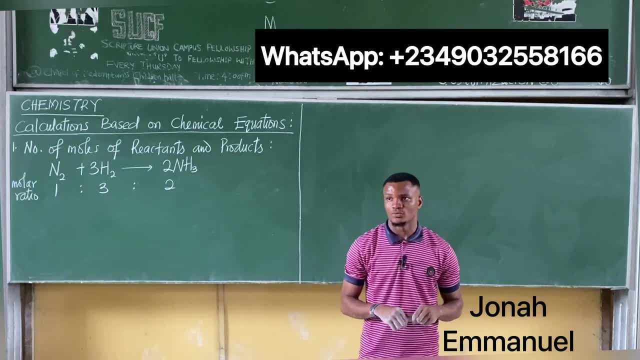 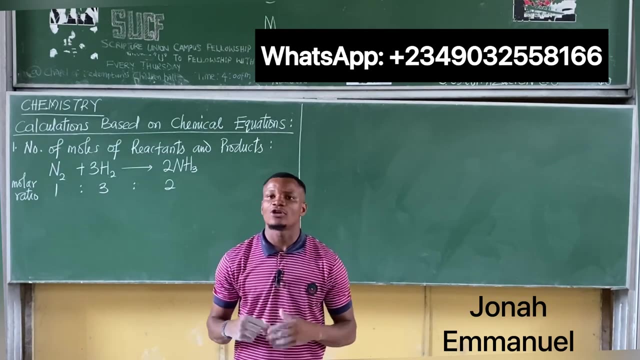 is 3, is 2, coefficients here is 2, so my molar ratio is 1, is to 3, is to 2, it's called a molar ratio. listen and listen carefully for every calculation that is involved in equations at your level, they will always. 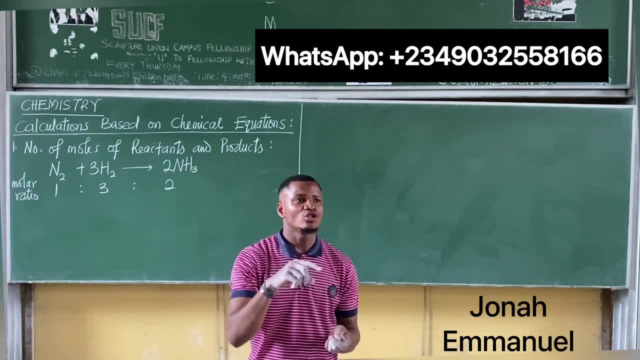 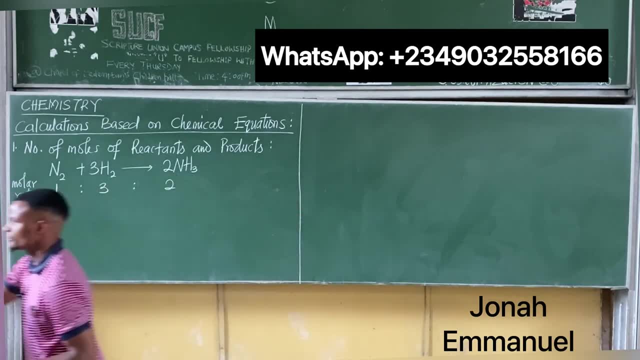 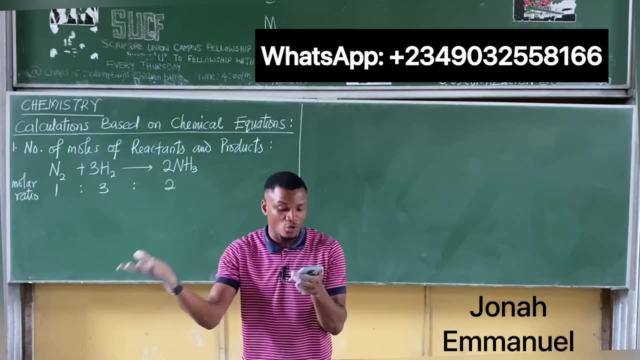 no matter the number of reactants and products, they will always give your focus to 2 to 2,. please check your question, please. your question says nitrogen combines with hydrogen to form a ammonia. okay, so what they said? how many were there? 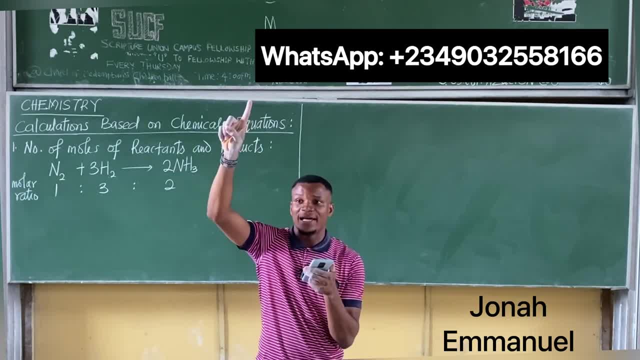 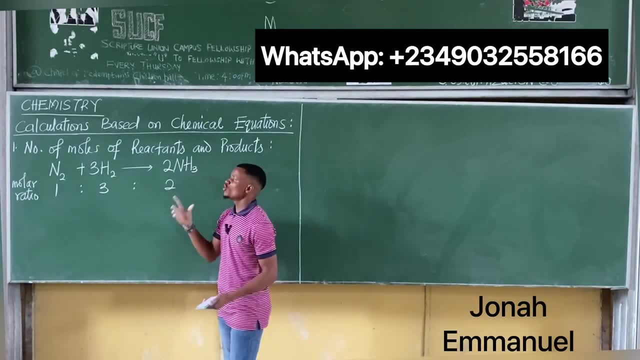 2. they mentioned hydrogen aha are required to do what there they said, those products. so observe that first of all, they helped us to form our equation. and I said: no matter the number of products and reactants in our equation, they will always narrow your mind to 2. 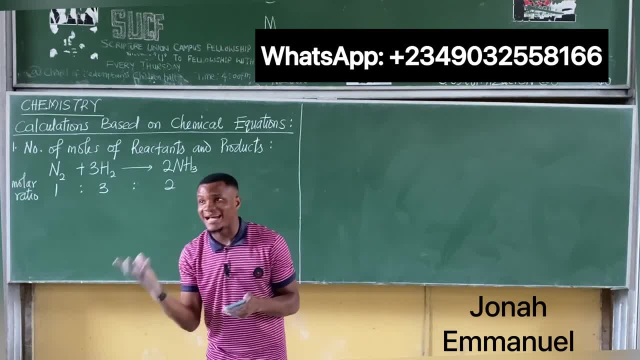 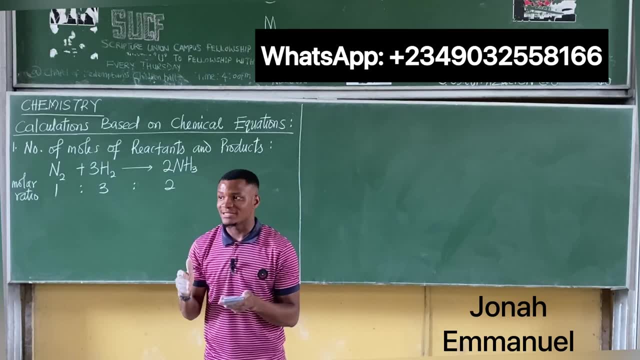 the 2 in this equation are what there 2, hydrogen and nitrogen. how many moles of hydrogen are required to react to what there? thereан� 300, and we not necessarily g or ers- to 100. 300 moves of what Nitrogen. So it means in this case: 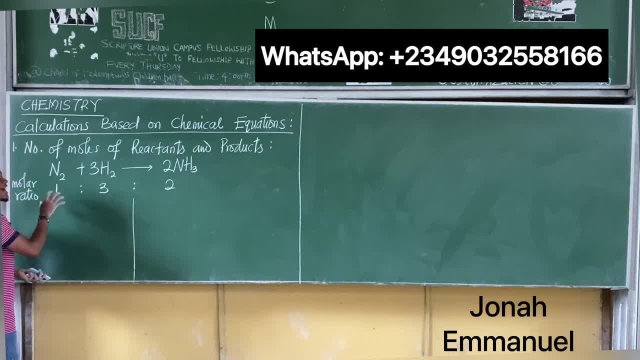 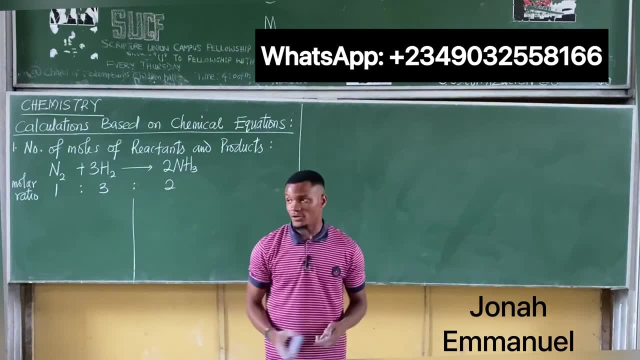 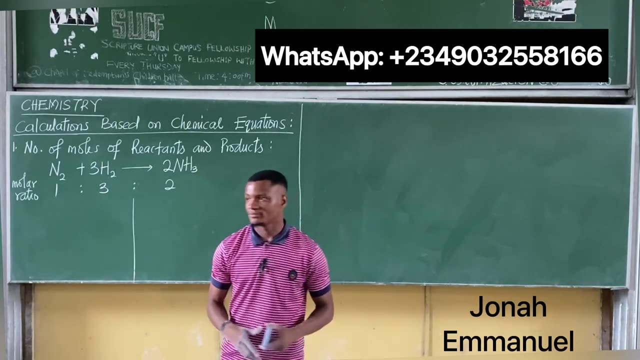 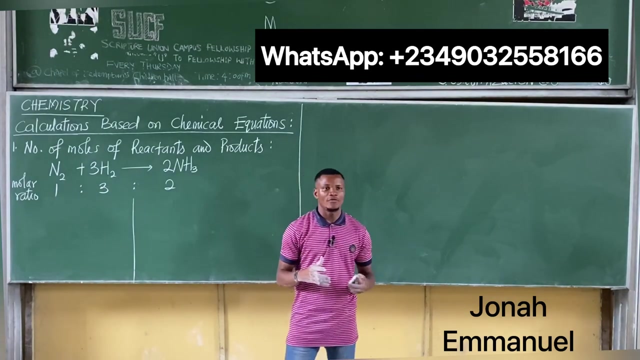 here, I'll simply narrow my focus towards hydrogen and nitrogen. Alright, if you are here, take down this statement. If you are here, take down this statement please, From the balanced equation of the reaction. from the balanced equation of the reaction. so see here one mole of. 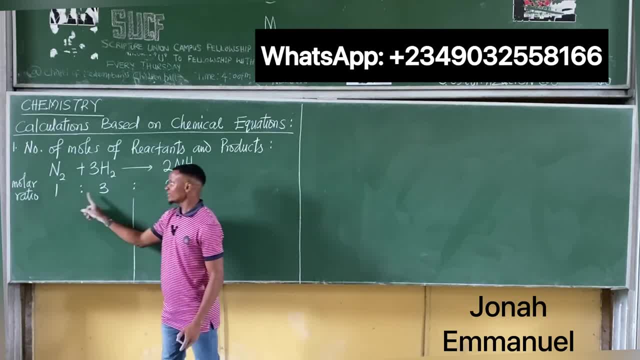 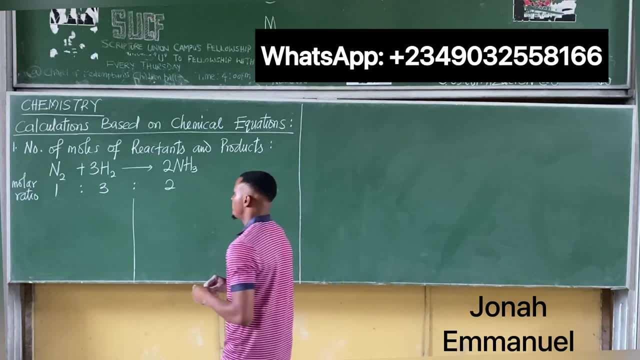 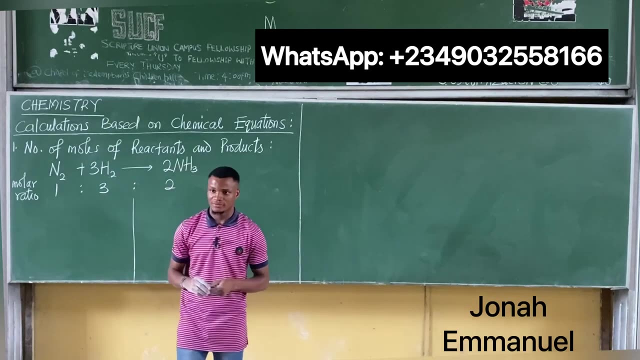 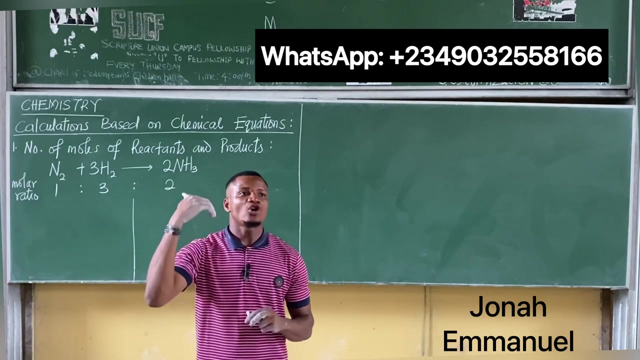 nitrogen is needed to react with three moles of hydrogen. You can see that From the balanced equation of the reaction, one mole of nitrogen is needed to react with three moles of hydrogen. We'll stop Let the amount of moles. they ask you how many moles of hydrogen? Let's call it x, unknown. Alright, Let the amount of moles of hydrogen, let the amount of moles of hydrogen required to react with 300 moles of nitrogen be x. So we don't know, let's call it x. Let the amount of moles of hydrogen required to react with. 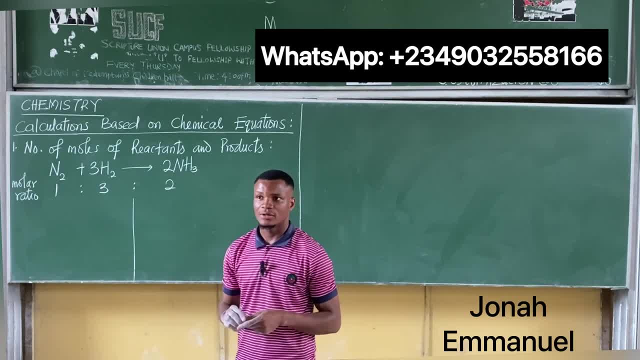 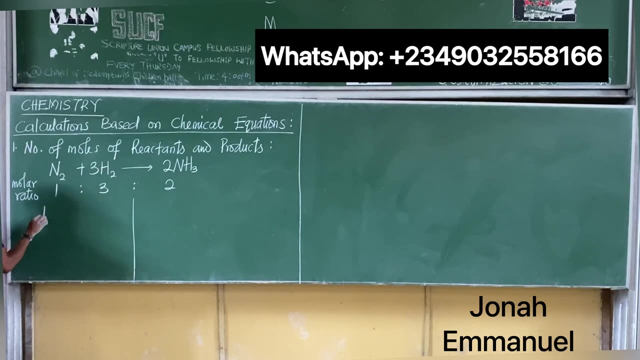 300 moles of nitrogen, be x, Hence. hence, if you don't look up this, so next up, I said, in all of this we'll focus on two, which in this case was nitrogen and hydrogen. So please, you do this From balanced equation of reaction. 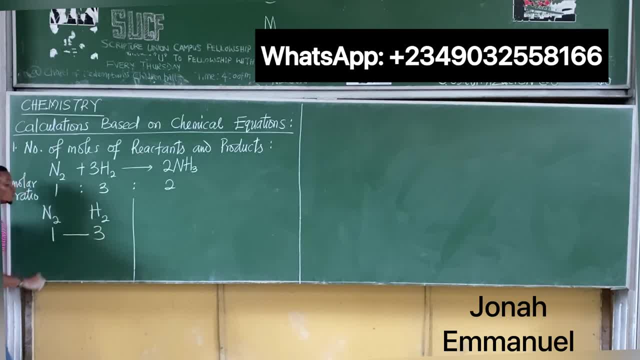 one mole of nitrogen is needed to react with three moles of hydrogen. We said, let the number of moles of hydrogen that will react with how many nitrogen there With 300.. We don't know how many of this would react with 300. 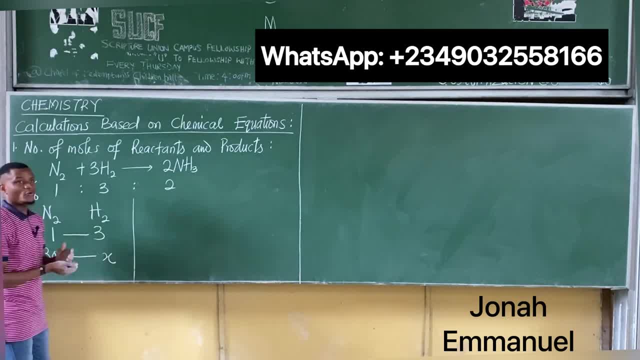 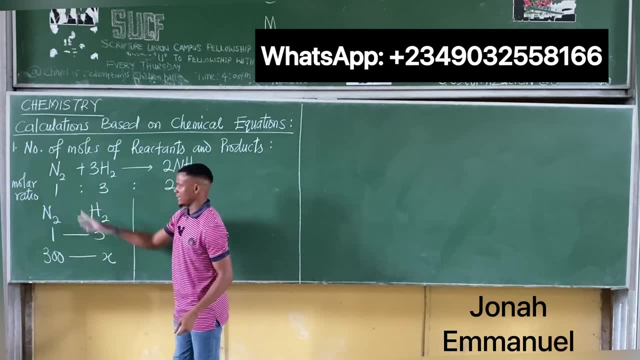 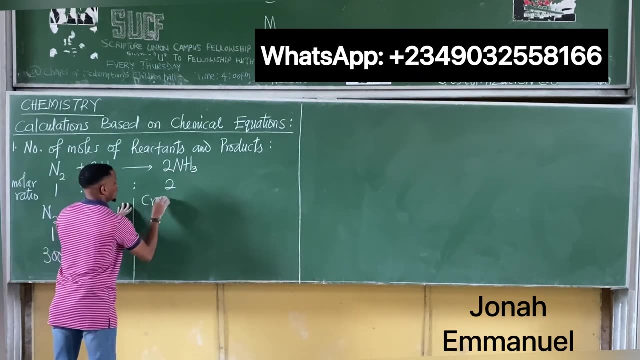 We call it x, let it be x. So the idea is always simple. You always have the two elements, The first one from your balanced equation and then the unknowns. That's this At this point, what next Cross multiplied? so I'll now cross multiply. 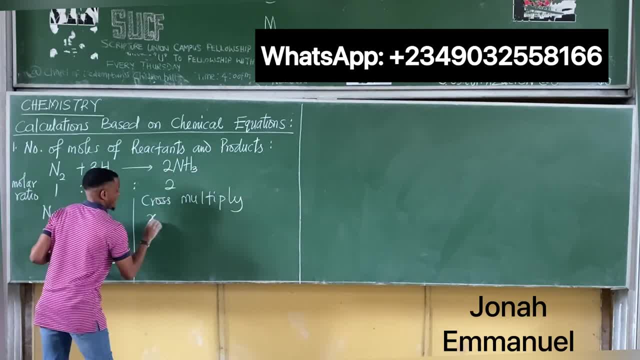 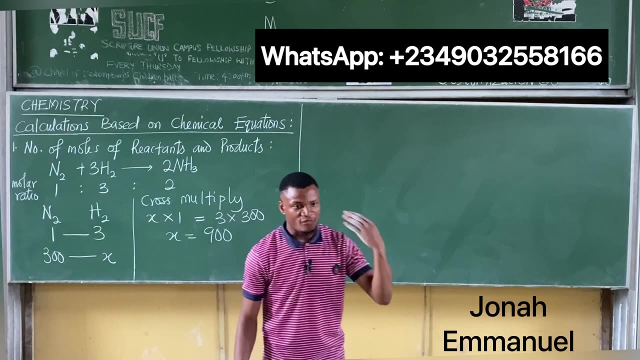 so I have x times 1. so x times 1 is equal to this times this 3 times 300. so I have that x is equal to 900. check: we said x represents what there number of moles of hydrogen. so therefore x is 900. 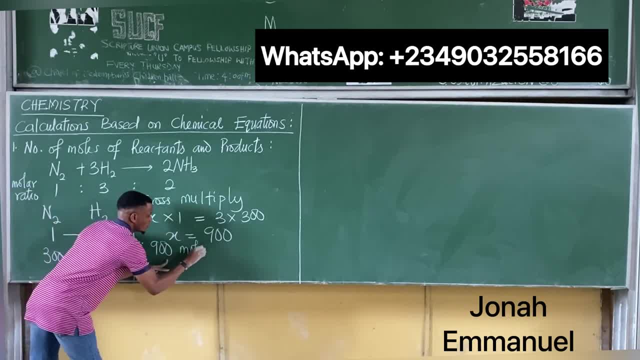 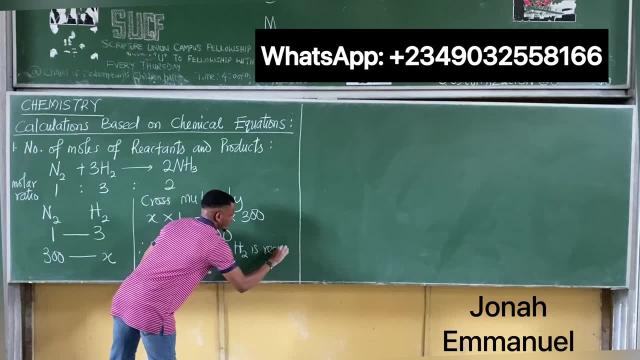 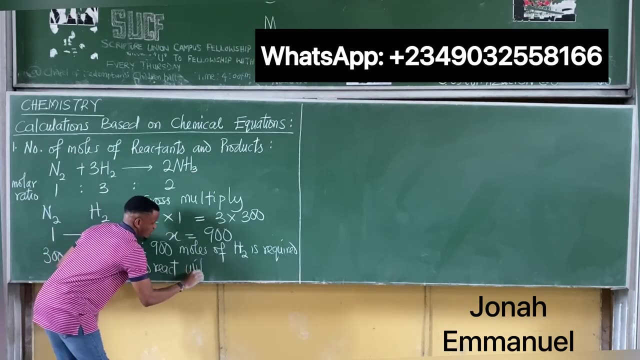 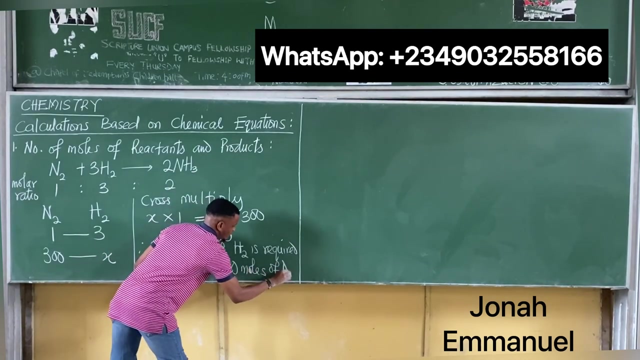 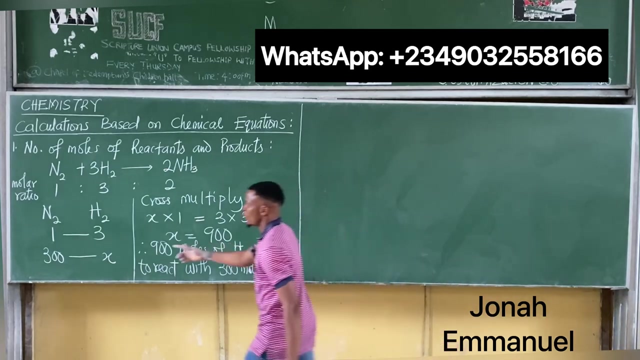 so, therefore, 900 moles of hydrogen H2 is required to react with to react with 300 moles of nitrogen. it is this simple. please, in all your distance, that will give you 2, 2. think of it. as to. the first line of equation will be from the balanced reaction. 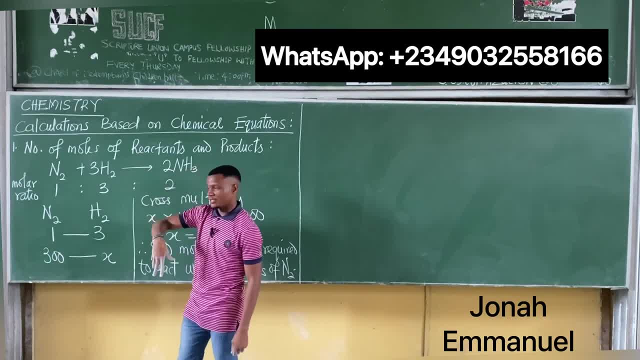 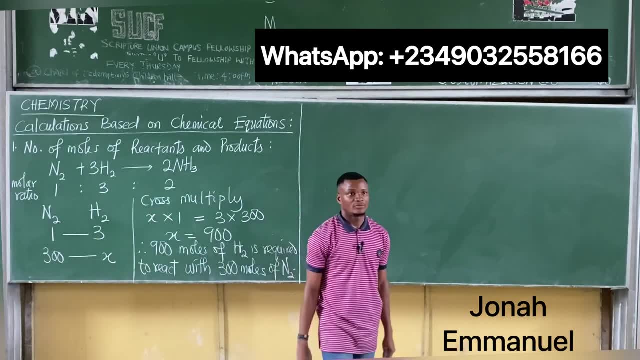 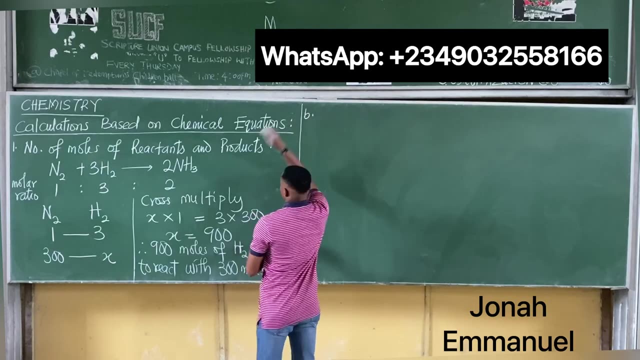 the second one now will now be from the question they said: how many of hydrogen will react with 300 of this? so cross, multiply and get x. it's simple. let's look at something much more complex. the first one is number of moles. 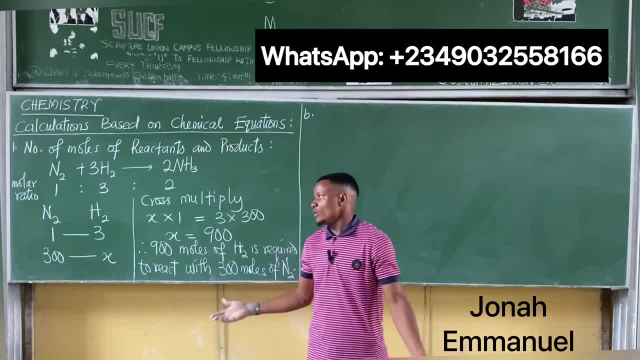 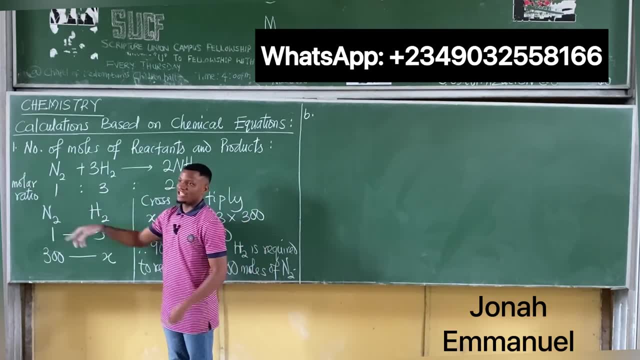 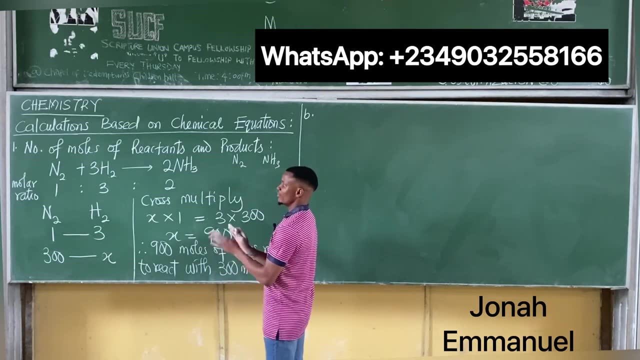 of reactants and products. they can still ask you how many moles of ammonia can be formed from 20 moles of nitrogen. in that case it becomes nitrogen N2 and ammonia NH3. first of all, get the molar balance 1 and 2. 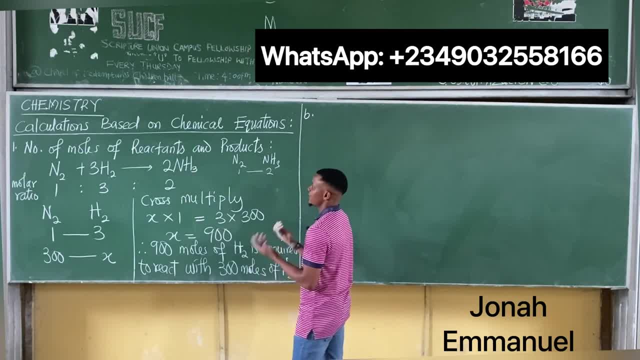 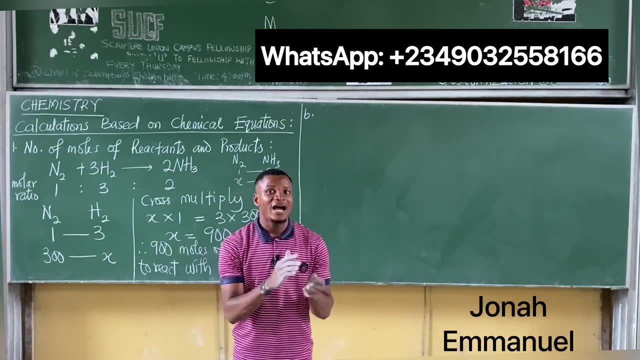 so 1 and 2, if they say how many moles of nitrogen x will be needed to produce 500 moles of ammonia, 500, so it's easy. it's easy, that's one number. 2, observe: in the question they said how many moles. 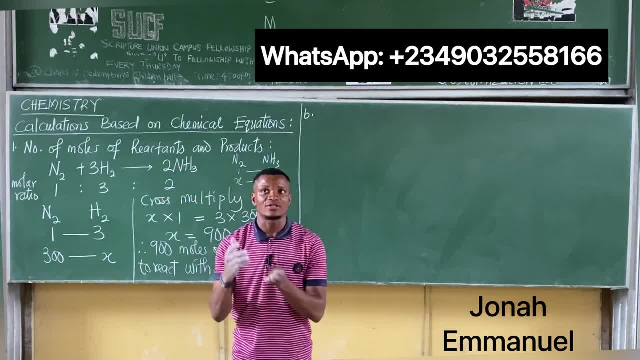 of hydrogen is needed to react with 300 of nitrogen. so it's like saying in my question they mentioned hydrogen first before nitrogen, but in my solving observe I wrote nitrogen before hydrogen. why I am following the sequence of the equation? 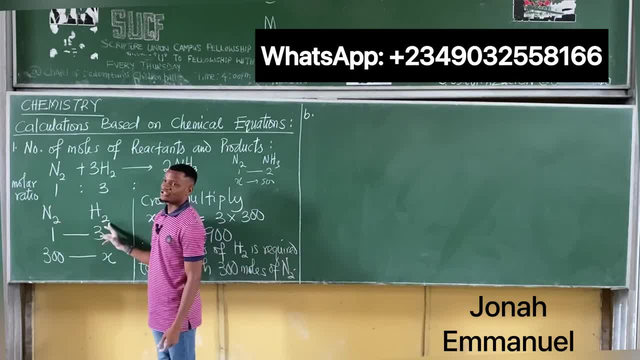 so, although they mentioned hydrogen before nitrogen, I wrote like this just so I can follow the equation: but what if you choose to swap it H2 and N2, is it wrong? No, but then it's not that proper. it's better you follow the sequence of so, even if they mention 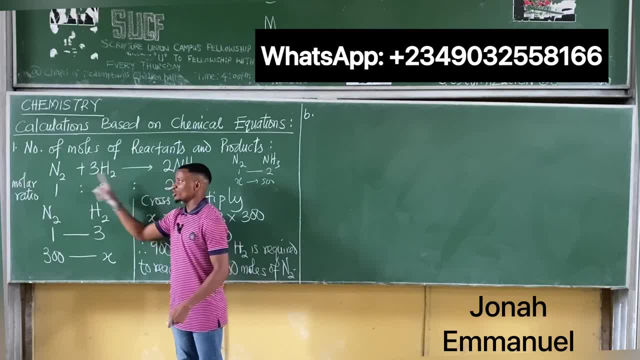 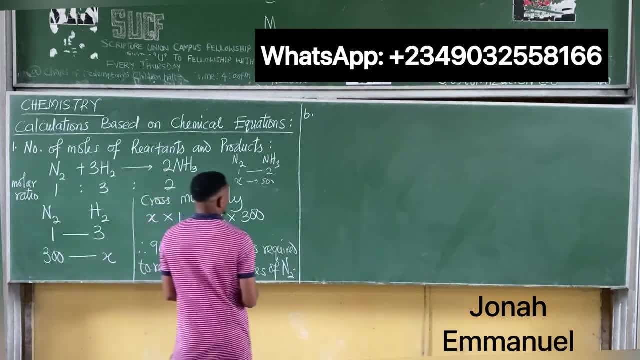 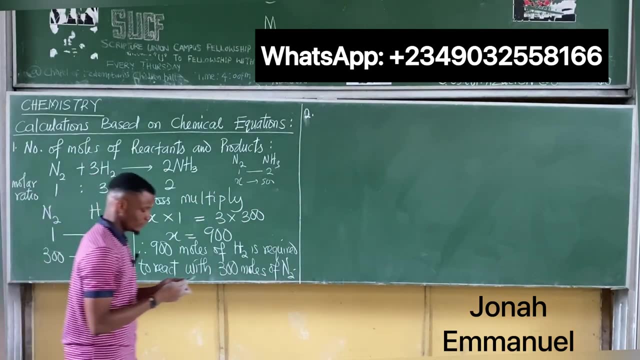 hydrogen before nitrogen for the fact that in my equation this one comes first. it's advisable this one first before this number 2. please sorry, that's my 1, number 2. number 2, mass number 2. calculation based on chemical equation. 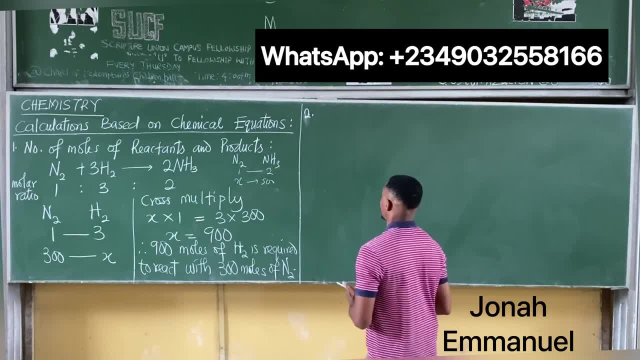 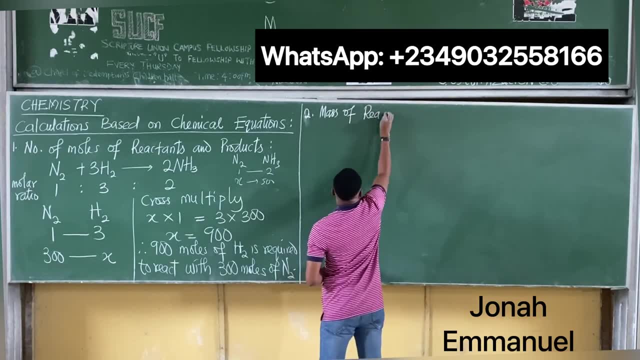 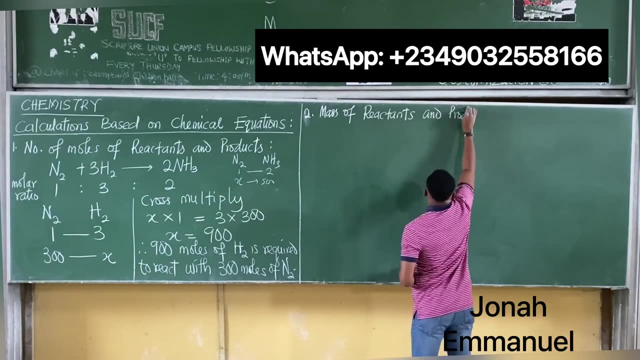 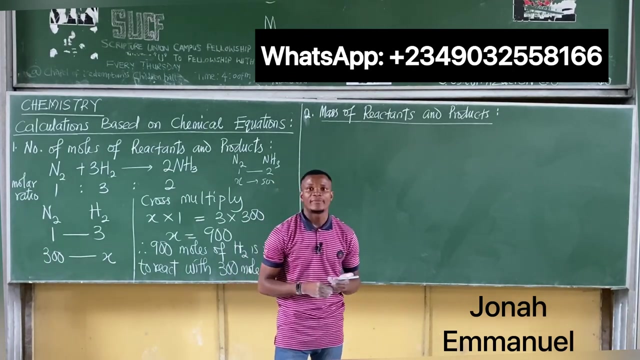 number 2: mass of reactants and products. bar 2: mass of reactants and products. you can continue in a given chemical reaction if you want to. or chemical equation: mass of reactants and products in a given chemical equation. take this down, please. what mass of oxygen? 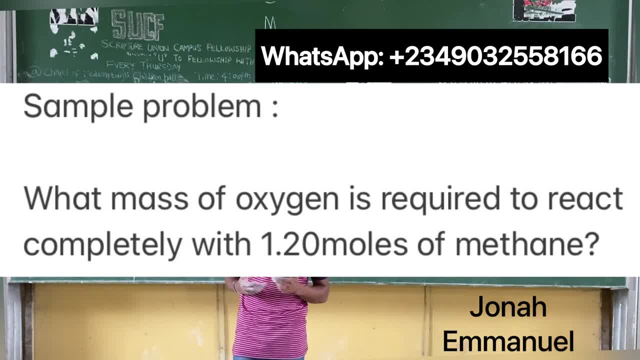 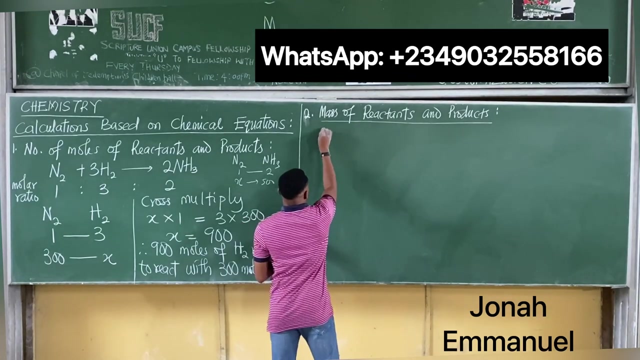 what mass of oxygen is required to what mass of oxygen is required to react completely? what mass of oxygen is required to react completely with 1.20 mole of methane? alright, so my question. we said methane. methane is what there? CH4 combined with oxygen, O2, to give you carbon dioxide. 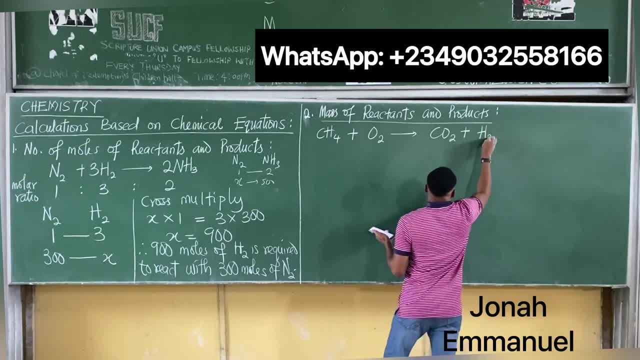 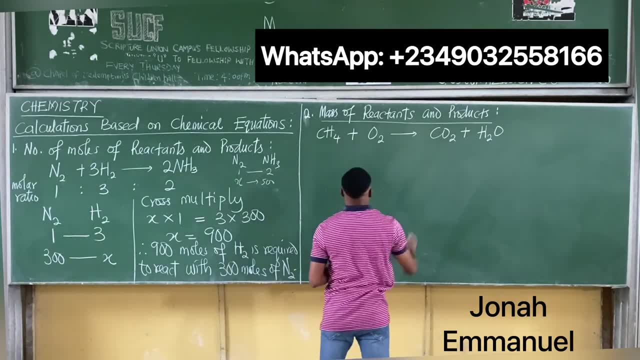 CO2 and water, H2O. are we still going to balance? so carbon 1 balance, hydrogen 4, I will have to add 2 here, 2 and 2, 4, ok, oxygen 2 here. oxygen here. this is. 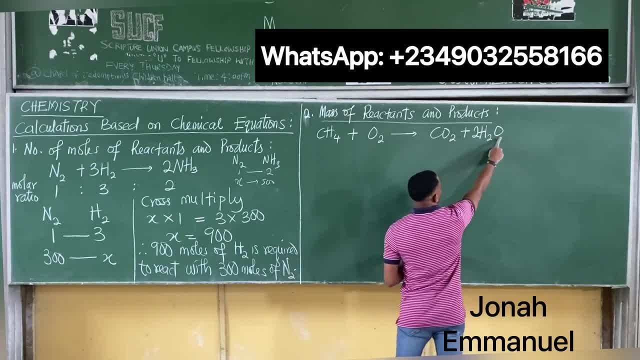 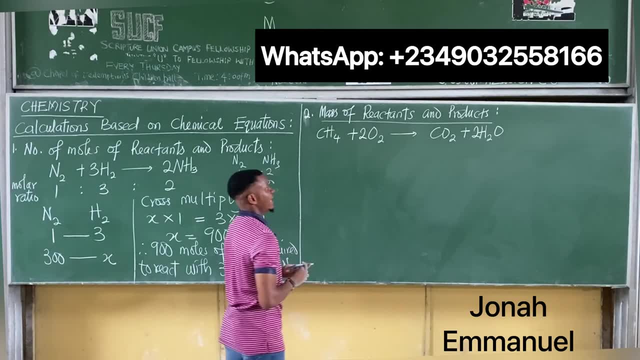 2 plus 2, this is 2 here, 2 times 1: 2, so 2 here plus 2 here, 4, this one is 2. I will add 2 here to make it 4, I now have a. 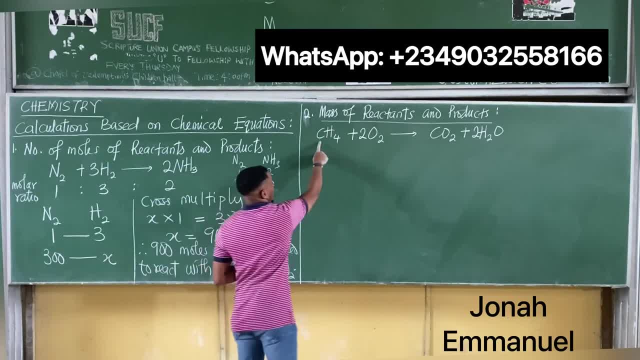 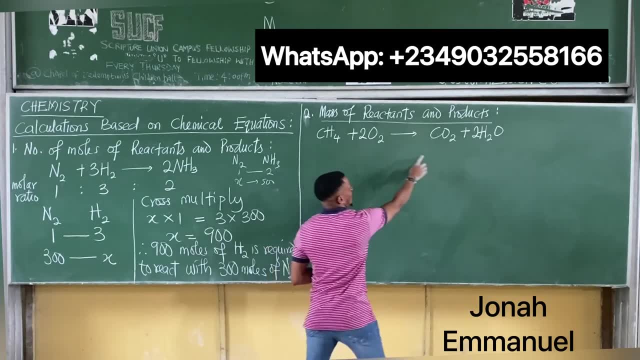 balanced chemical equation, please check: carbon is 1: 1,. hydrogen is 4, 2 times 2, 4. oxygen is 2 times 2, 4, this is 2, 2 times 1, 2, so 2 plus 2, 4, it's a balanced. 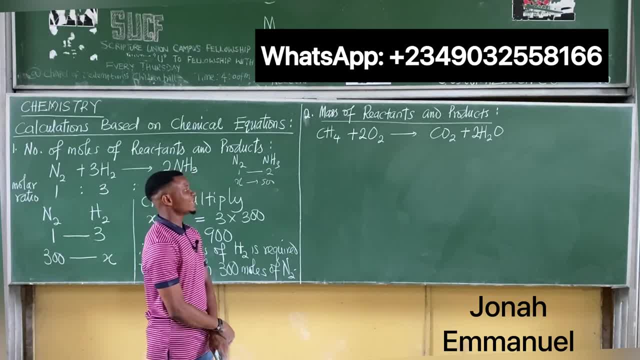 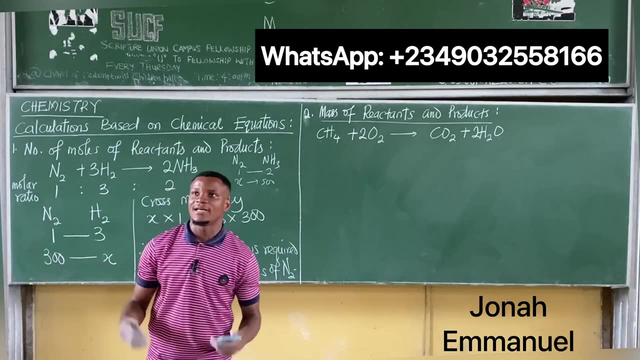 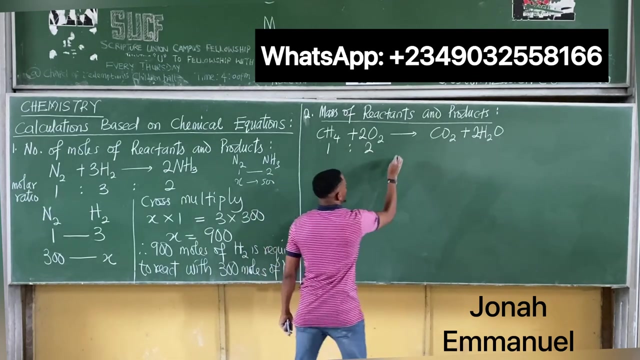 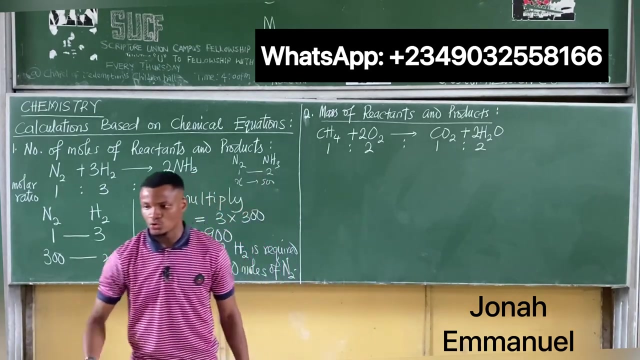 chemical equation. next tax: molar ratio. I've said molar ratio is as easy as whole number coefficient. Here is 1, is 2,. here is 2, is 2,. here is 1, is 2, 2. My molar ratio is 1 is to 2, is to 1. 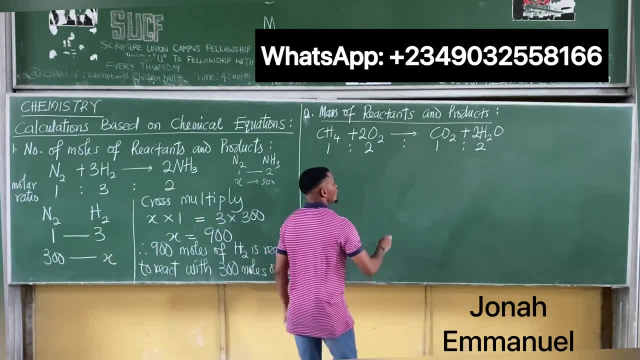 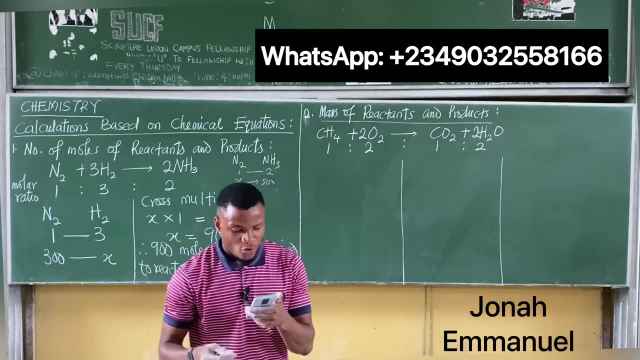 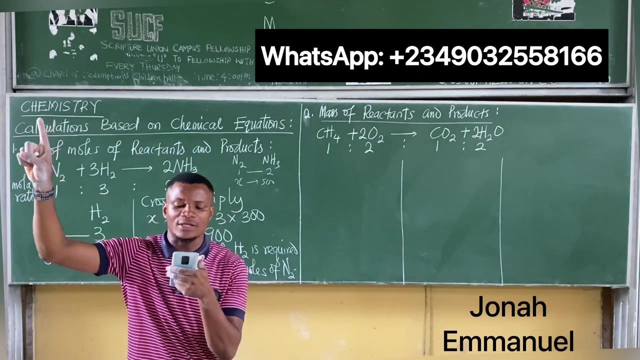 That's my task. Next up, I said check For every question. they will narrow your attention to 2 particular, Perhaps 1 reactant or 1 product. Please check In your question what kind of work was considered, What mass of oxygen. So oxygen number 1 is required to react completely with what? 1.20 mole of methane. So oxygen and methane are my 2 focus. Alright, So Your statement please From the balance equation of the reaction: 1 mole, 1 mole of methane, Will react with 2 moles of oxygen. You can see here From the balance equation of the reaction. You can write it down: 1 mole of methane Is required to react with 2 moles of oxygen. Let the number of moles of oxygen Require to react with 1.2 moles of methane, The X. Let the number of moles of oxygen. Require to react with 1.2 moles of methane, The X. Hence, Of course. Hence, we'll have this one. first, Methane Bx. Now what we will do it: methane, CH4, oxygen O2, okay, this is 1 and 2, notice that, notice that when I'm writing, 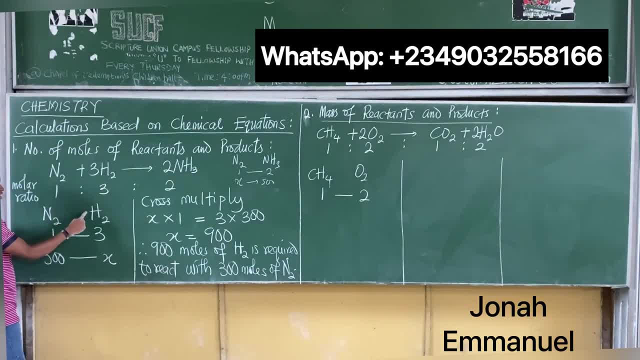 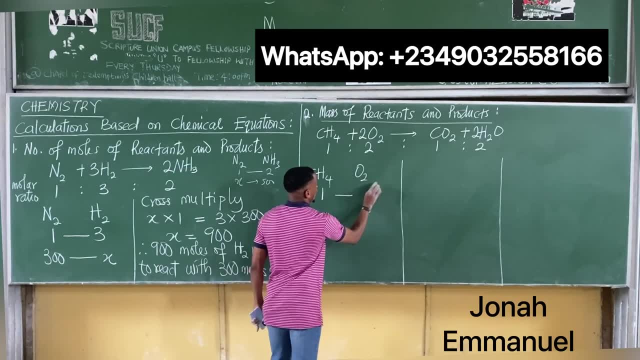 these ones here. I don't put this one, so I didn't write 3H2, no, just H2, leave out the 3, these 3 comes here. so in the same vein I'm having 1 and 2, we said number of. moles of oxygen should be X, so X of this becomes 1.2 moles of methane. I have this, of course. find X cross. multiply this and this X times 1 is equal to this times this 2 times 1.2, so X is equal to 2.4 moles of oxygen. now check your question. it didn't. 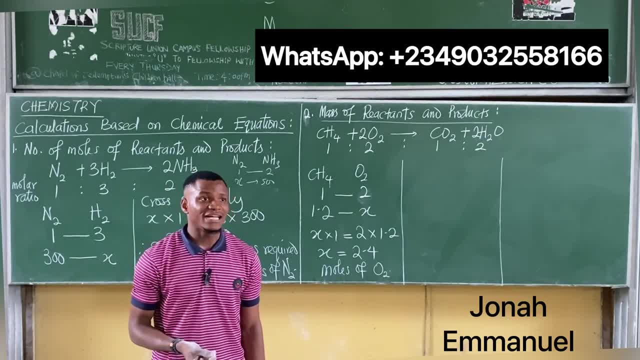 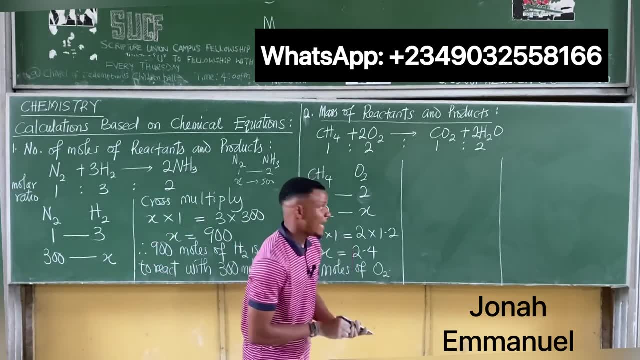 ask you for how many moles of oxygen. check It. asked you for what there Mass mass. I have mole of oxygen. can I find mass? Yes, How Now recall that will say that what there mole is equal to what. 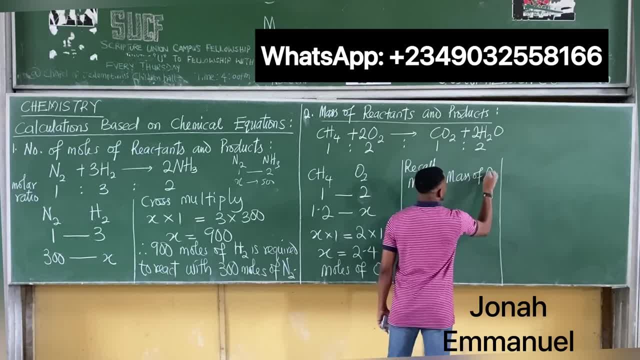 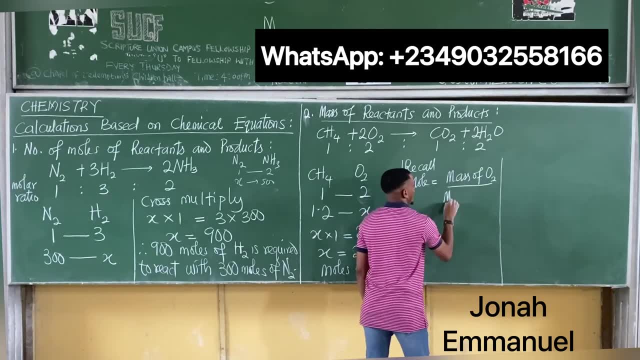 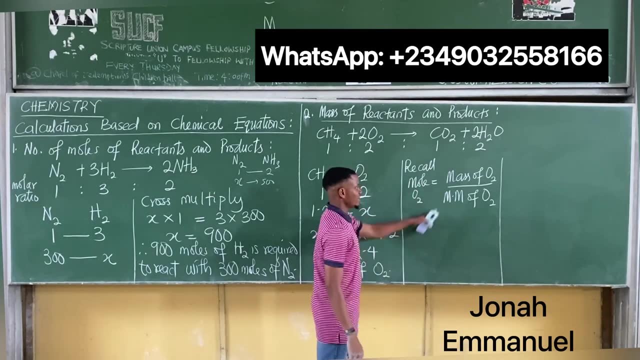 Mass, so mass of O2 all over. I'm writing this at mm because of space in yours. write molar mass, so molar mass of oxygen, So mole of oxygen. Oxygen is equal to the mass of oxygen all over molar mass. please, this is molar mass. 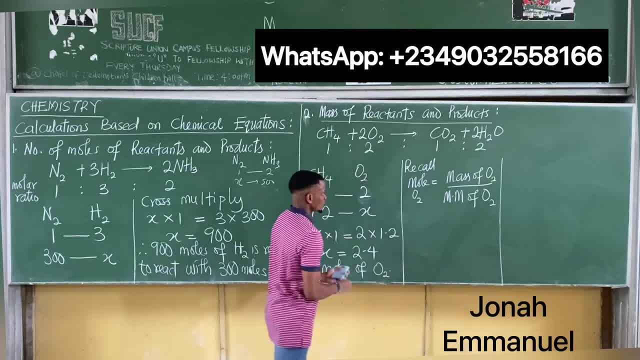 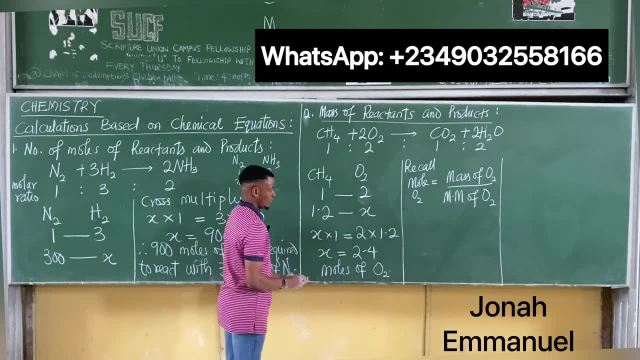 write in full. I'm trying to save up space. Alright, what do we have? We already have the mole of oxygen, which we've calculated as what? 2.4,. oh, mole, not molar mass, please. yeah, 2.4 mole, alright, so I'm having 2.4 mole. 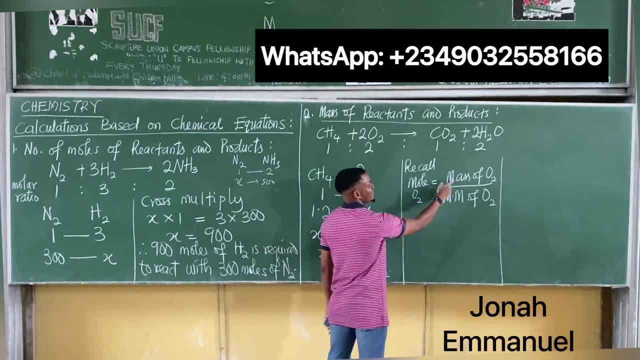 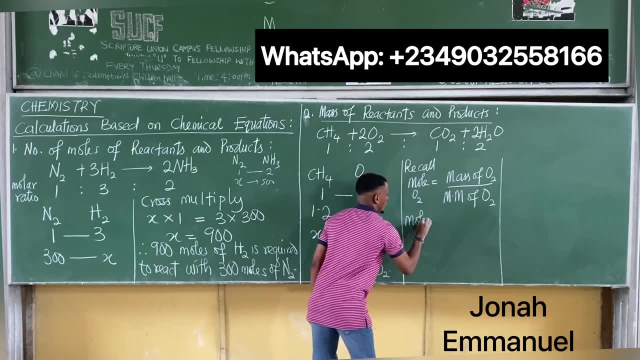 of oxygen. here I have this. I'm having to find mass. of course, first of all I have to find what there? Molar mass. let me get this value: Molar mass, molar mass of oxygen- O2, will be equal to for oxygen. what's the atomic? 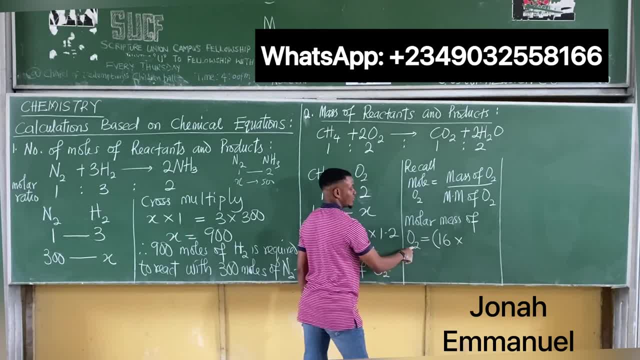 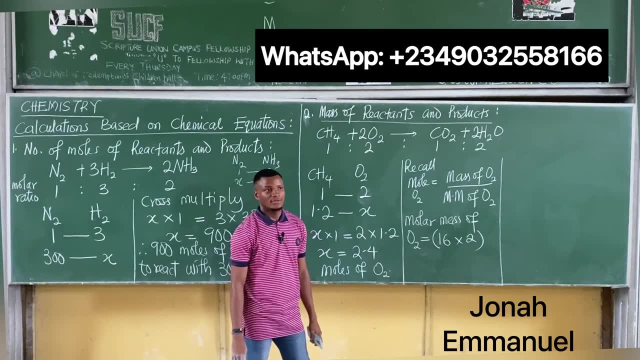 mass 16 times how many atoms there Times 2 atoms, please. 16 is the atomic mass of oxygen. it's a constant. please. 16 is the atomic mass of oxygen. it's a constant. so that's equal to what there. 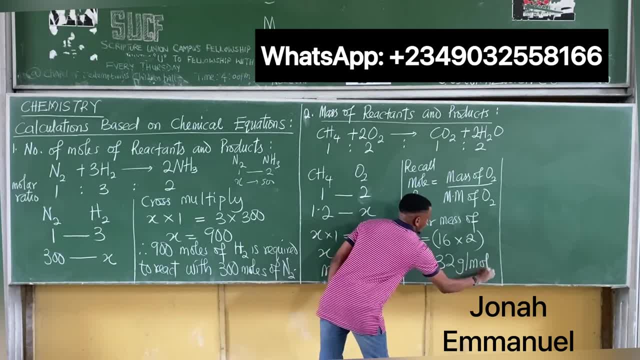 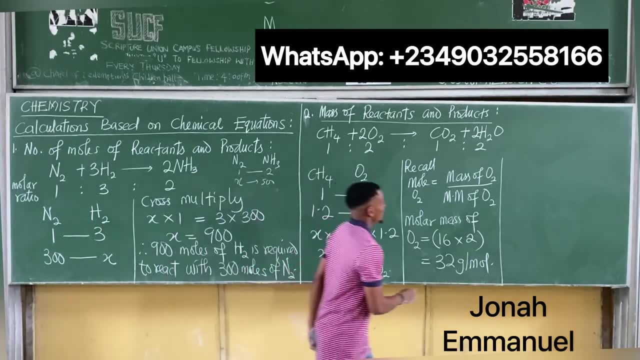 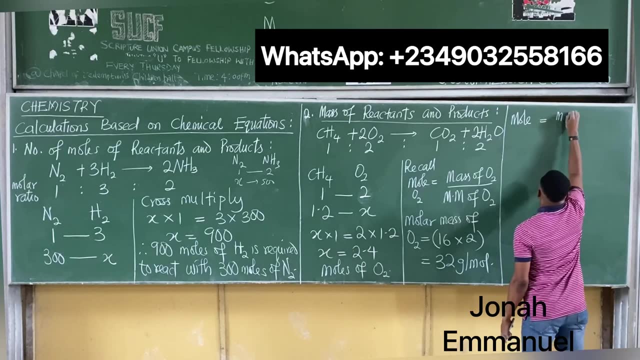 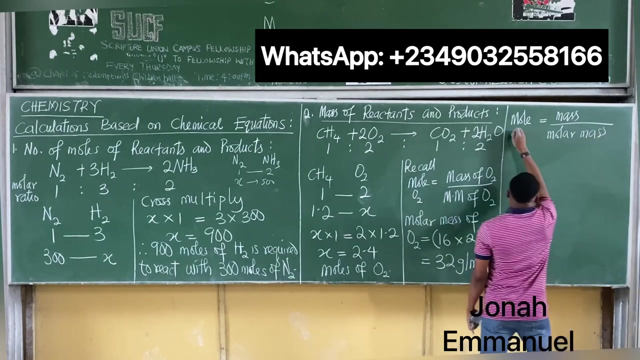 32., 32., 32., 32.. If I've gotten molar mass and I've gotten mole, I can now find mass. of course, from here we know that mole is equal to mass all over molar mass. so look up please. if 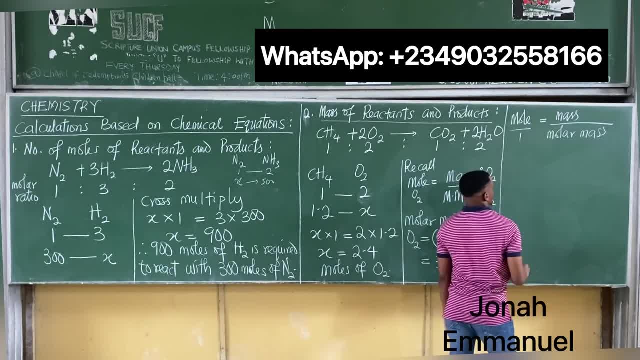 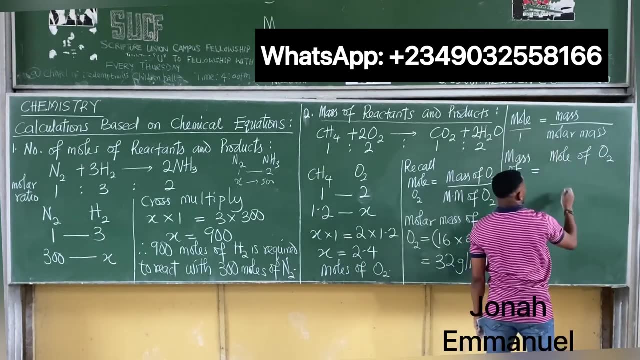 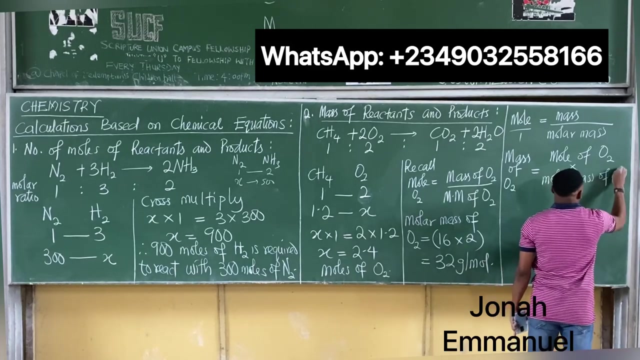 I'm to get mass. it becomes mass times 1, that gives you mass. so hence the mass of oxygen- O2, will be equal to the mole of oxygen. so mole of oxygen, this one times, this one times molar mass of oxygen. so hence, mass of oxygen is equal to mole of oxygen. 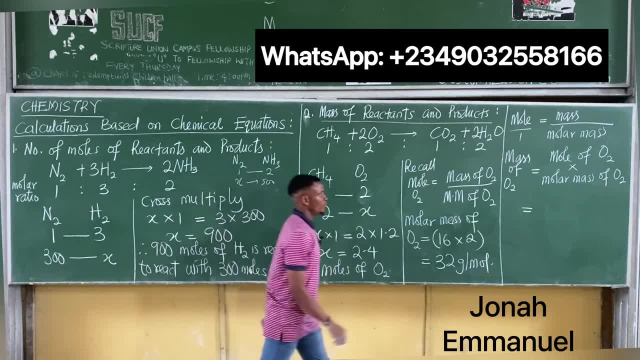 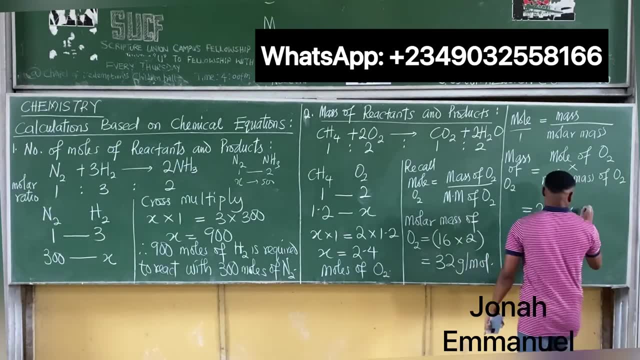 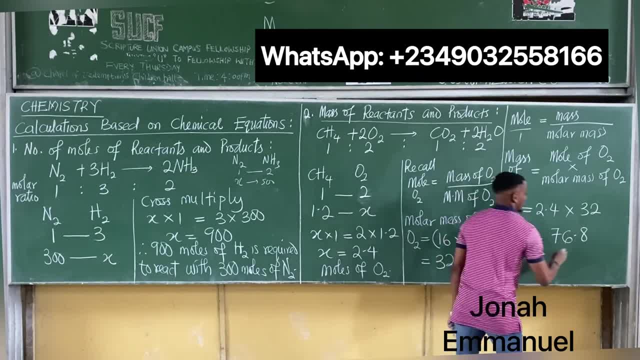 2.4., 2.4., 2.4., 2.4.. This one here, this one here, this one here. actually, I have this one which is 0.2, times molar mass of oxygen. we've calculated this. that's what. 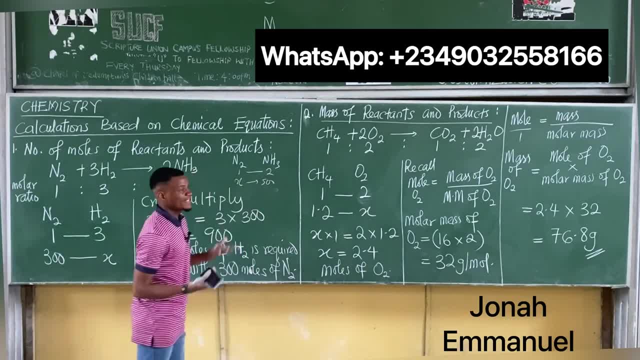 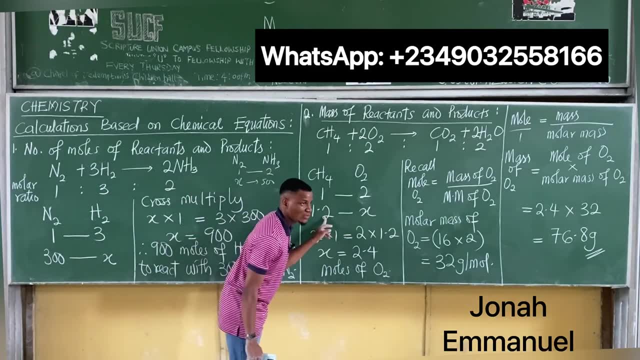 32. 32.. Please multiply this. what do I have? 0.8.. 0.8, what Mass? Mass? Yeah, It's in gram, so please see the difference. These two are similar. 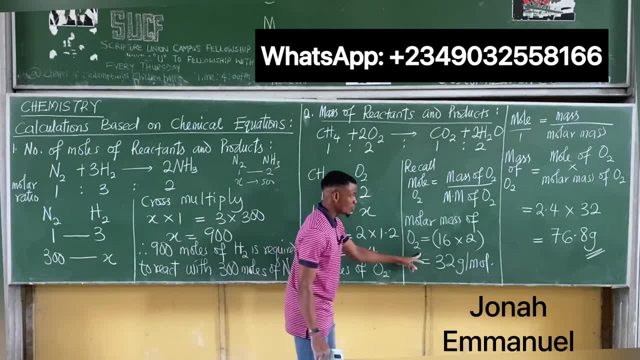 The difference is that for this one, I'll find mole and stop. they ask me for mole, so find mole and stop the mole. you still have to find what's there- mass- by using this formula. so mass is just simply mole, which is this. 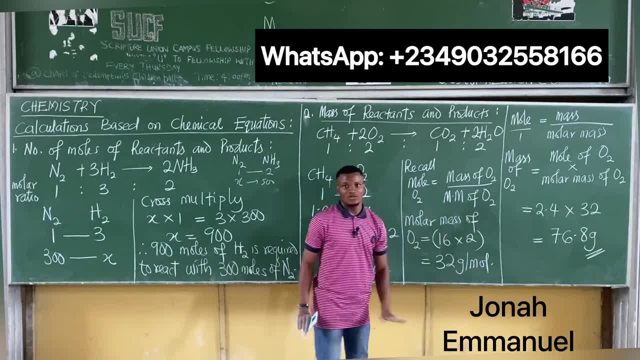 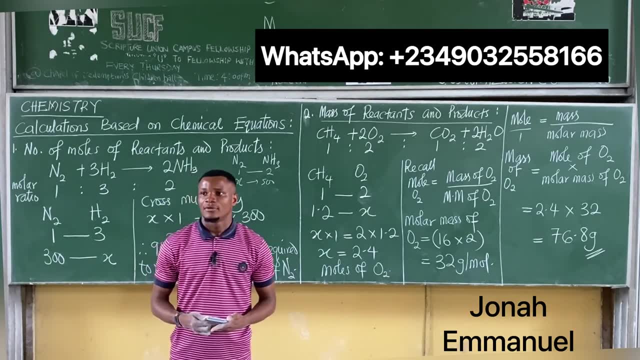 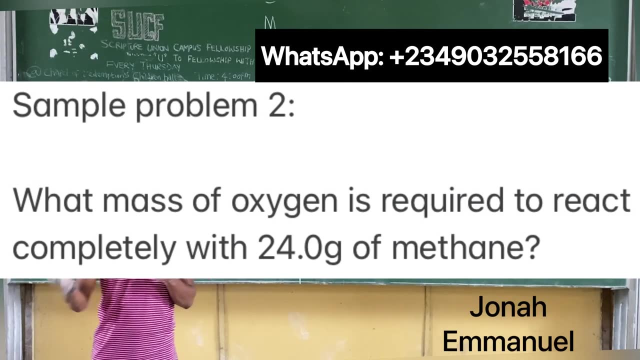 times molar mass, which we've gotten this and that, so there's no big deal. no big deal. so mass equals to mole times molar mass. any questions please? so I said example 2, I said what mass of oxygen is required to react completely with. 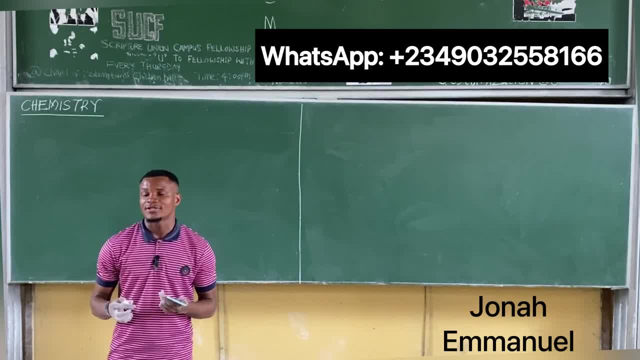 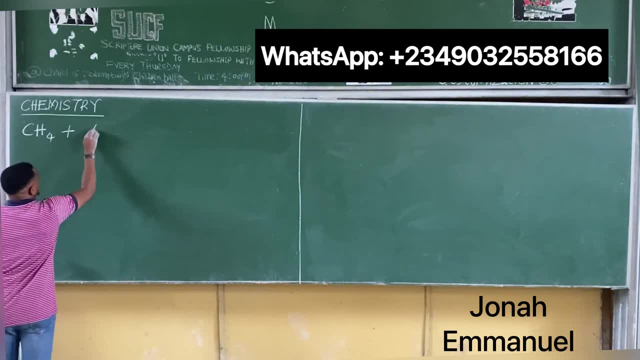 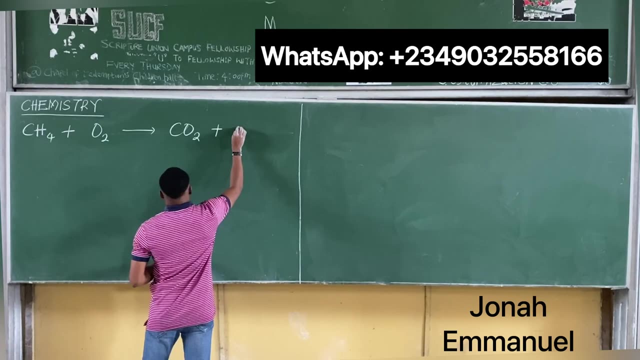 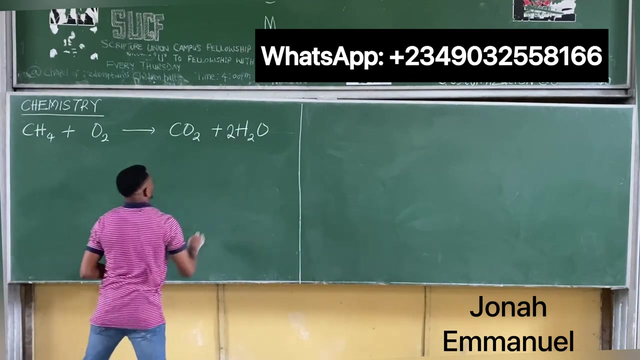 24.0 gram of methane. of course, the same equation of reaction: that methane, CH4 combined with oxygen, O2, will give you carbon dioxide, CO2, and water, H2O. ok, balance up. we had 2 here and we had 2 here. molar ratio was: 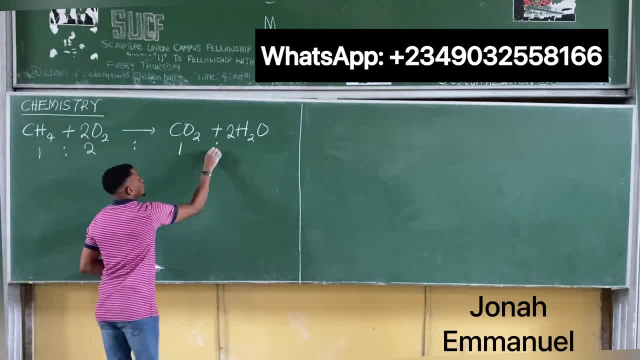 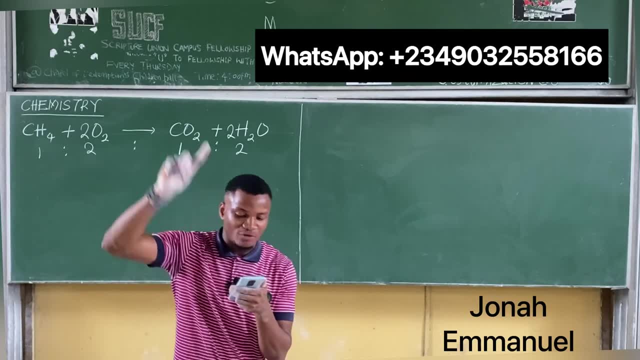 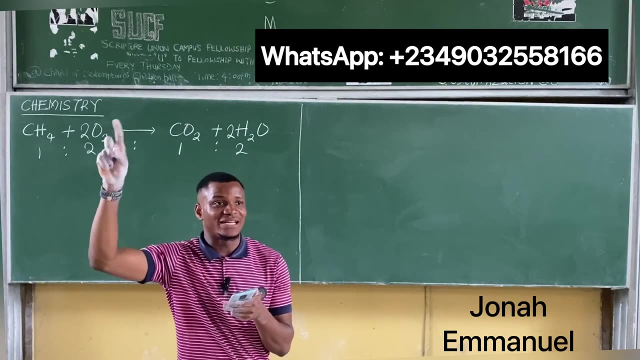 1 is to 2 is to one is to two. next up, pick out the two important things there. they said what mass of oxygen? so number one: oxygen is required to react completely with 24.0 gram of methane. so oxygen and methane are the two important thing there. so my look up, please, look up, please. my first thing is: 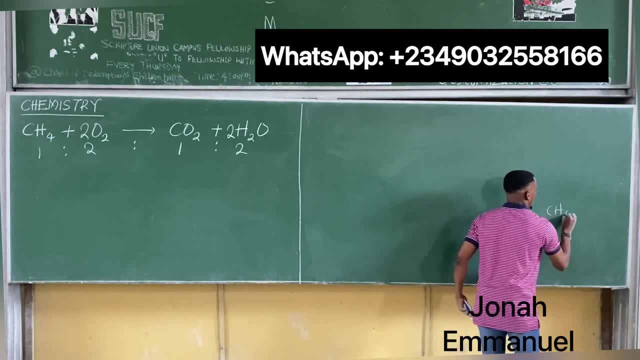 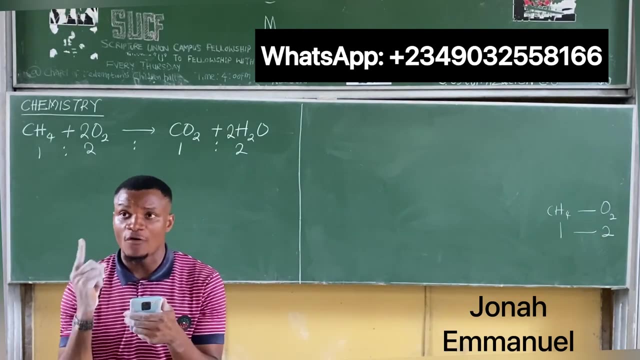 this. i'm given methane, ch4 and oxygen o2 from my balance equation. this one here is one and this is two. now observe something. observe something. in this case, it said what mass of oxygen. so i'm going to find mass of oxygen. okay, it's required to react completely with. now observe, they gave. 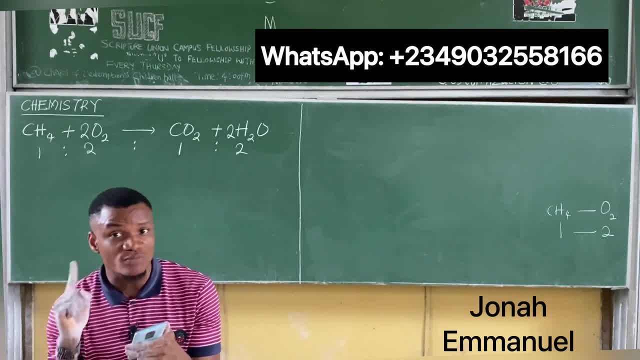 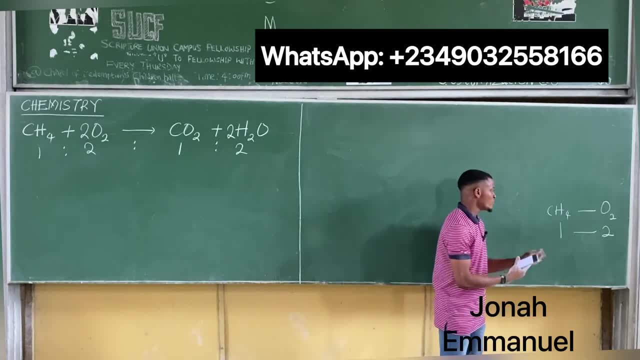 you what they're: 24.0, what they're gram, not mole, not mole you usually in our servings we need more. check out this example there they give us more for this 1.20 mole, but in this case they give us what now mass, no longer mole. so what's the task? 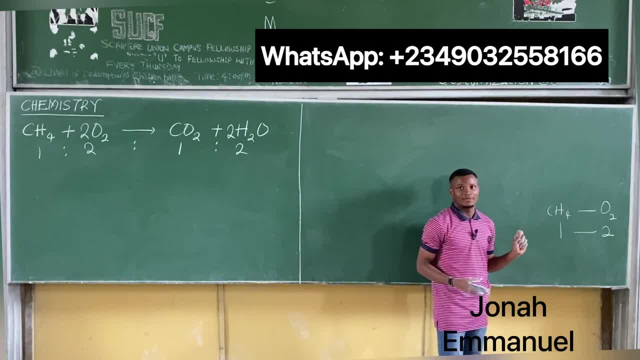 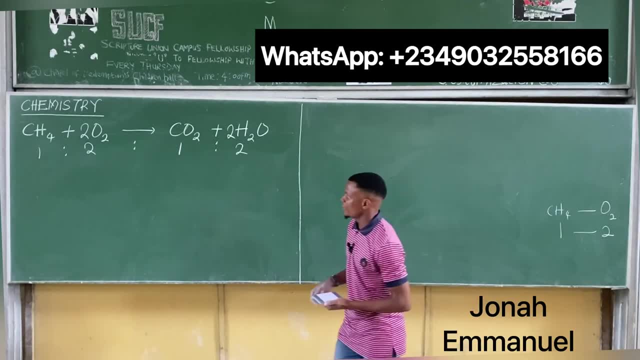 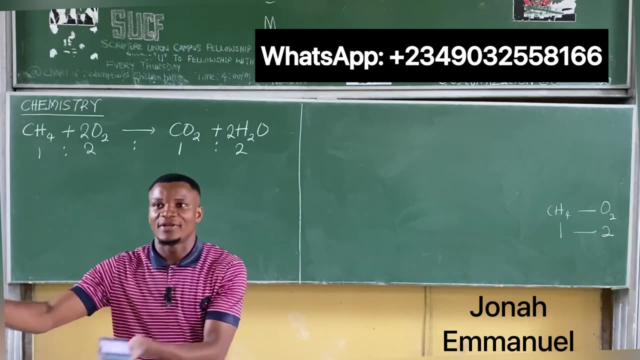 convert that mass to what there mole. that's the task. convert that 24 gram, which is mass, convert to mole first. that's the first task. all right, so my first task will be: depends on how you want to start. so let's start properly, right from the balance equation, from the balance equation that we want to convert is, is and than. 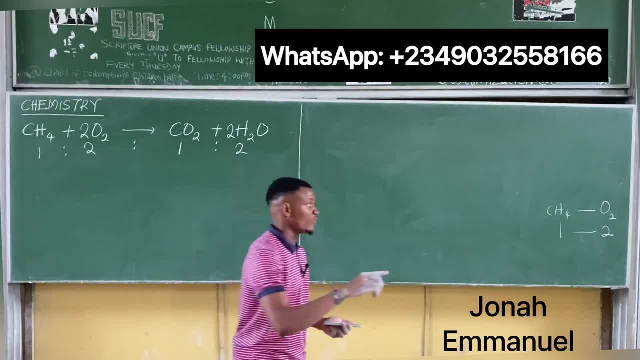 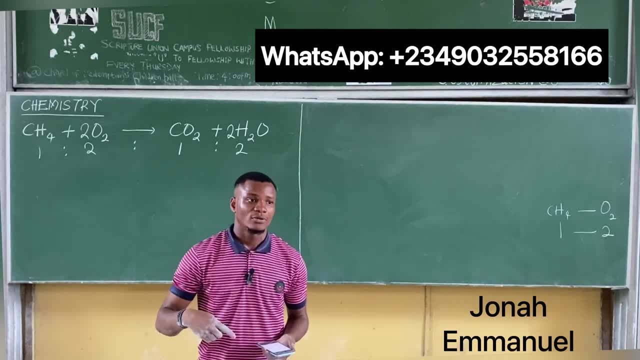 ketchup. difference between chewcheese. ideally the best way. record is sweet from the balance equation. okay, hold on, hold on, hold on. start this way, now we would have to come back. was that before all, zero gram of methane from mass to badly little bit the reason? 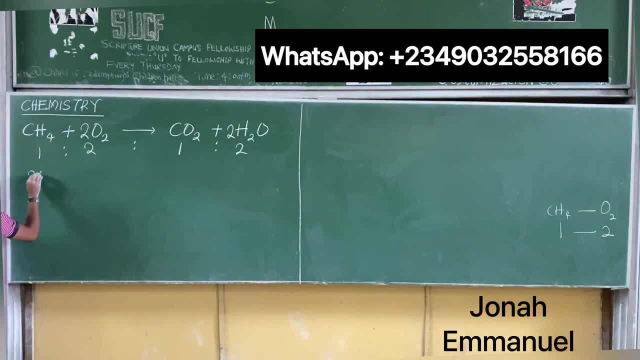 coating, but since just the 4.0 ground or anything. chq moon João, what do we know? when I God, move is equal to mass all over molar mass. So look out please. If I have mass of methane, all I have to do is to first of all get what there. 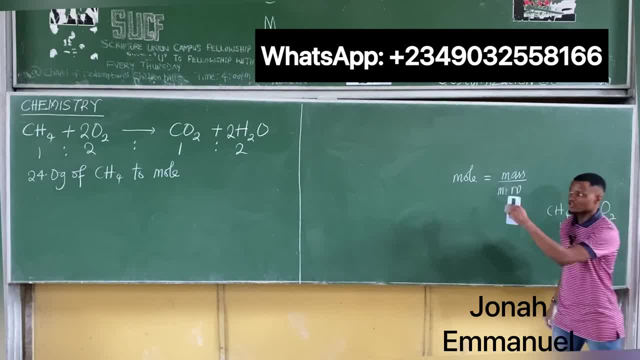 Molar mass of methane, So I can get more. So my task would be the molar mass of methane. the molar mass. the molar mass of CH4 is please for CH4, what's the molar mass For carbon? how many there? 12 plus hydrogen. 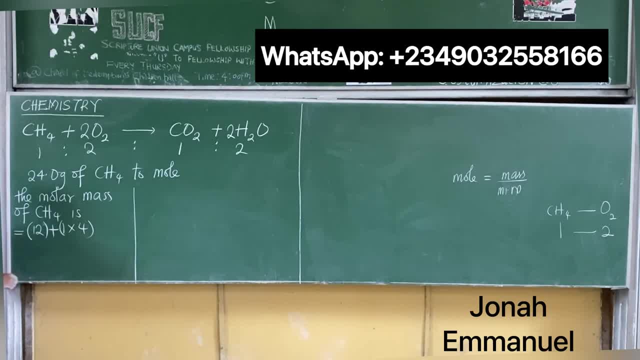 1 times 4, please. Atomic mass of carbon is 12.. Hydrogen is 1 times I have 4 hydrogen. So that's equal to 12 plus 4, that's equal to what there? 16 gram per mole. I'm calculating molar mass. 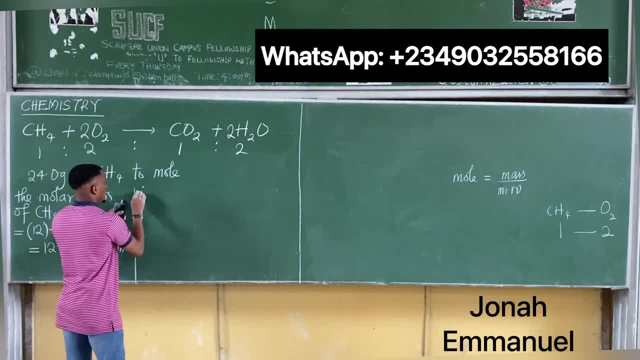 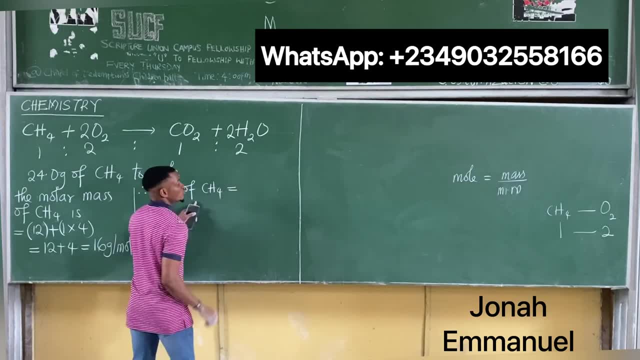 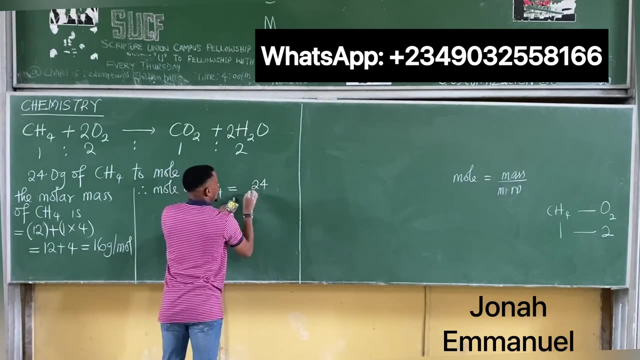 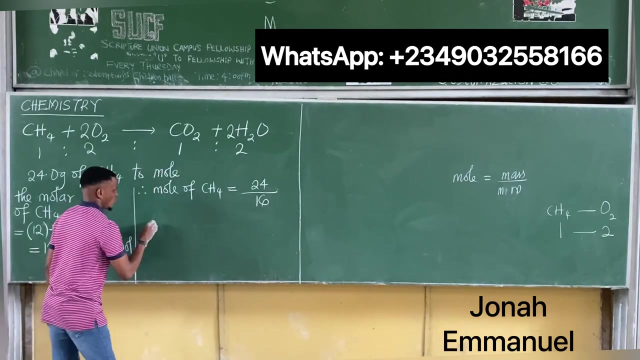 measured in gram per mole. So therefore, therefore, I can now find the mole of CH4, which is equal to, we said, mass of CH4, which is this one here: 24, all over molar mass of CH4, which is what? 16.. Alright, So what's the mole there? 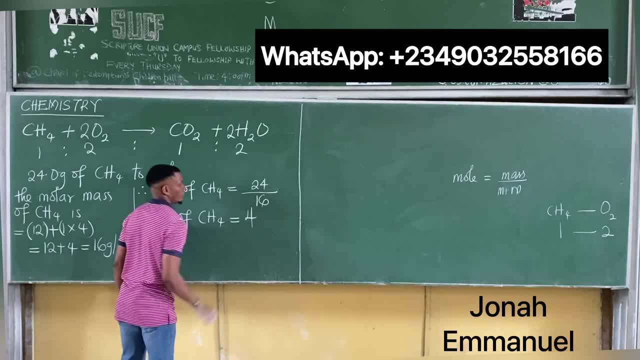 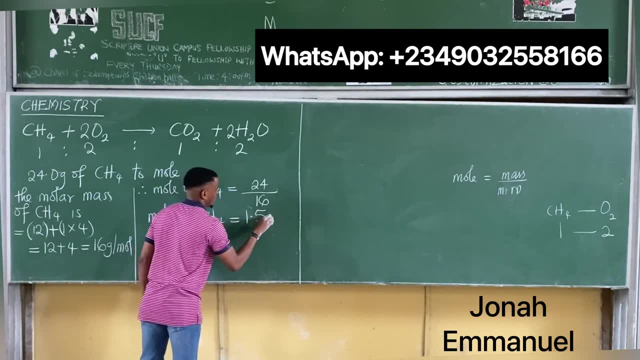 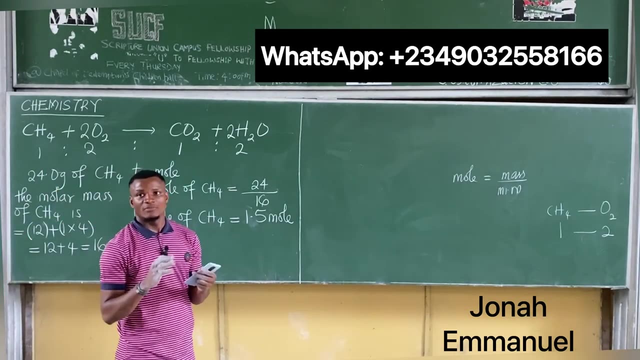 What's the mole there? Sorry, 4.1?. That's equal to 1. 1.5. what there Mole? So I have 1.5 mole. So it's a bit tricky, but please try to listen and get it. You know why I converted in this case. 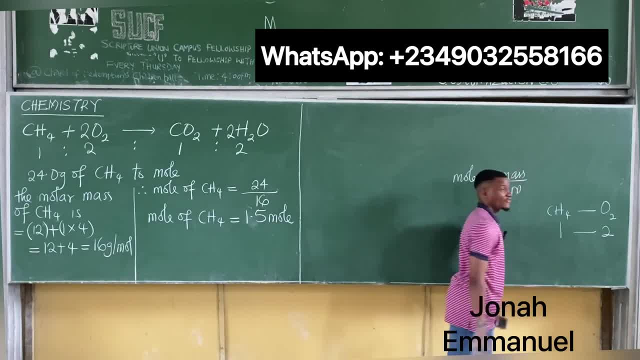 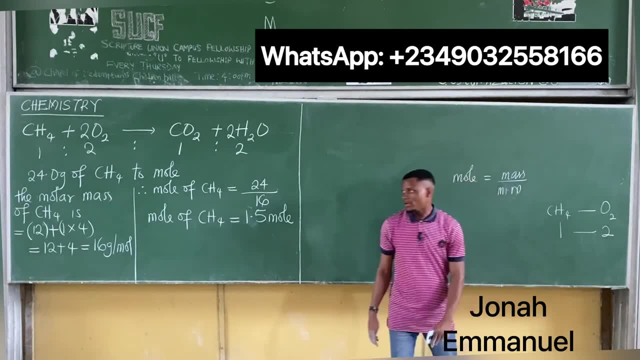 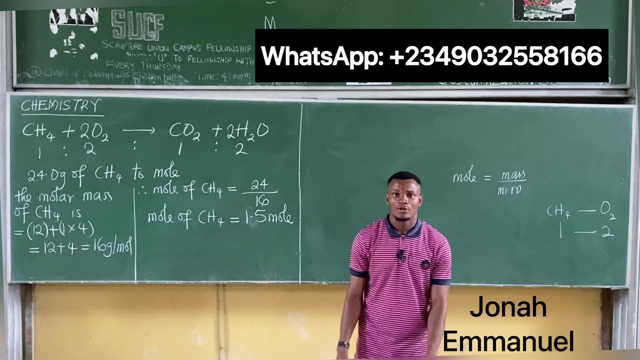 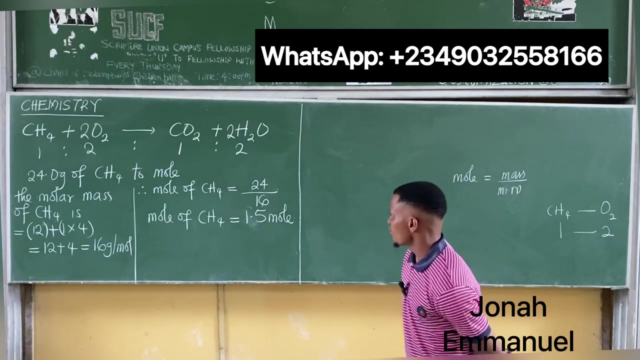 Because I'm supposed to work with mole, not masses. Instead of giving me mole. instead of giving me mole, you give me mass To convert the mass to mole first. Alright, So if you are here, let's proceed. let the number of, let the number of moles. 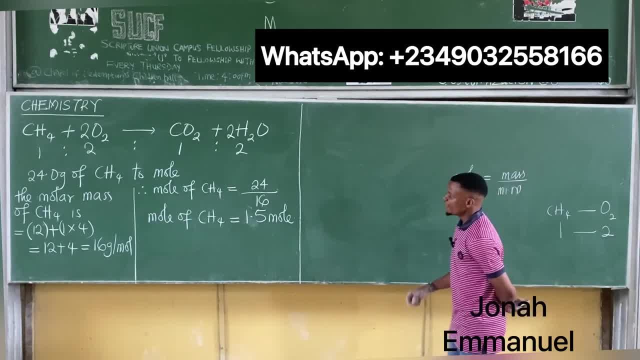 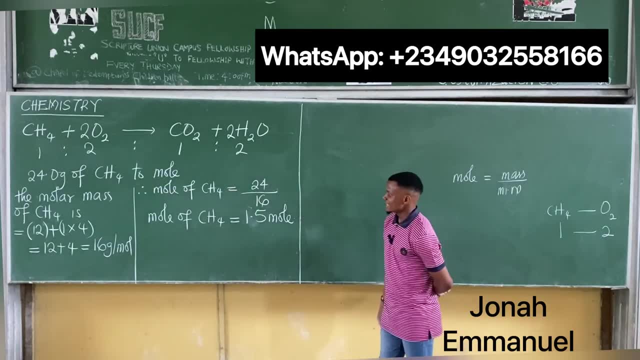 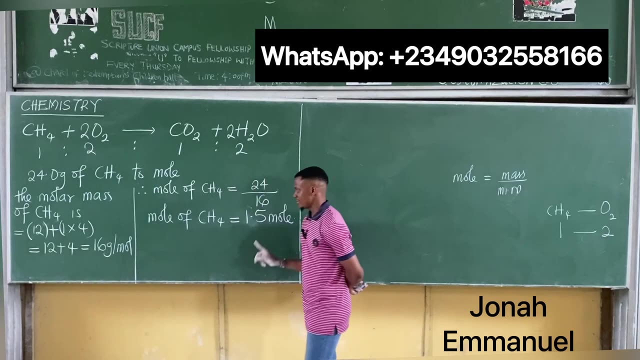 you work with. this is called molar ratio. let the number of moles of oxygen. let the number of moles of oxygen that will react with this one here now will not successfully convert the mass from here to mole. So we can now say this: Let the number of moles of oxygen that will react with 1.5 moles of methane be X. Let the number of moles of oxygen that will react with 1.5 moles of methane be X. Hence, hence this one first, methane, CH4,. 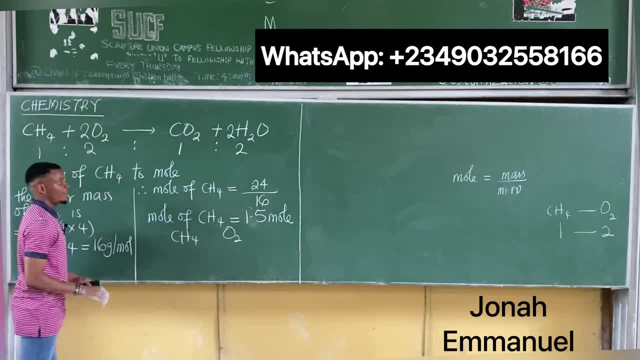 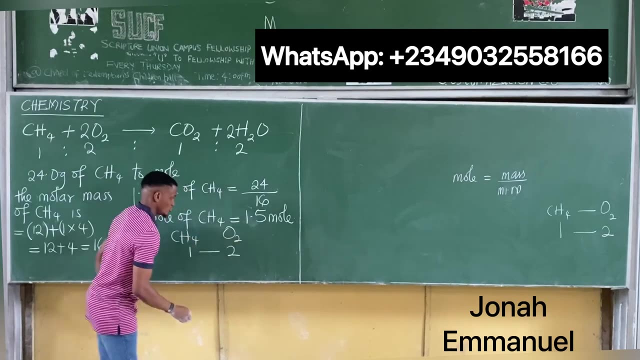 CH4, oxygen, O2.. First of all, mole ratio from balance equation 1 and 2.. So 1, 2.. Next up, moles as given. I wasn't given mole, I was given mass, I converted the mass to mole and I had this. So hence, 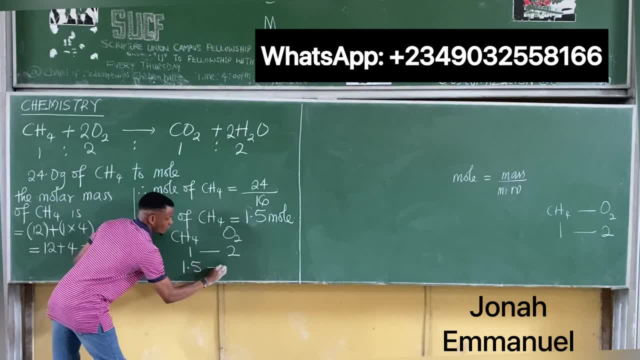 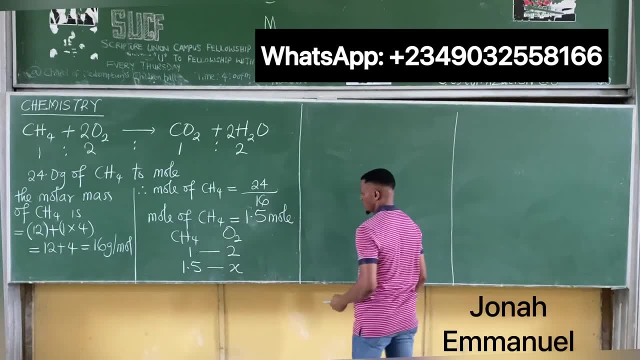 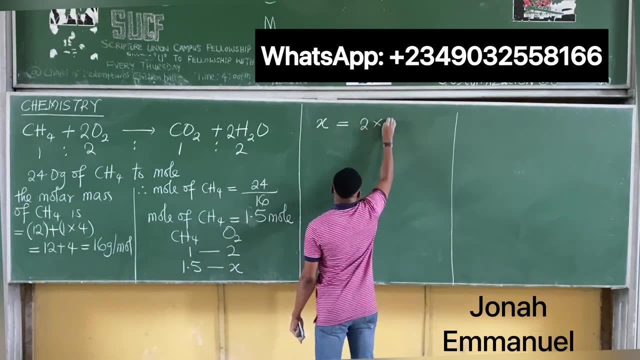 1.5 of the methane will be equal to X. So let's get X Alright. So simply, X times 1,, which is X, is equal to 2 times 1.5.. So X is equal to what there. 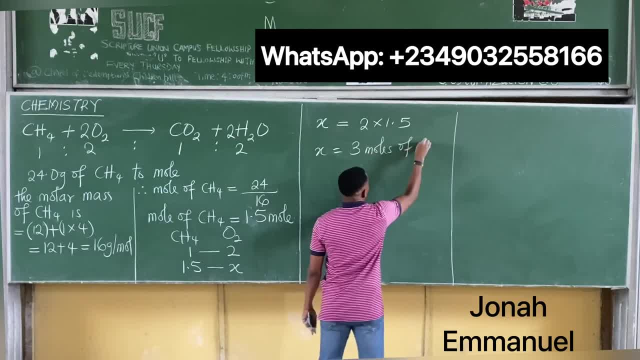 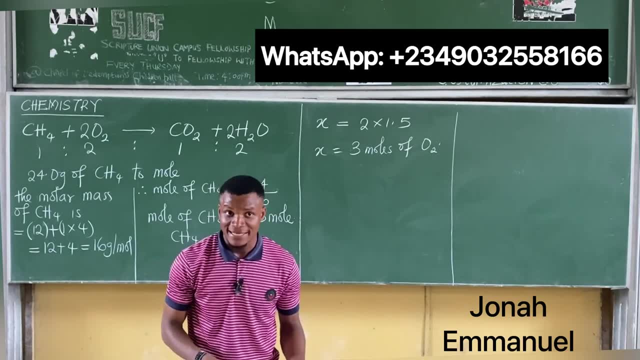 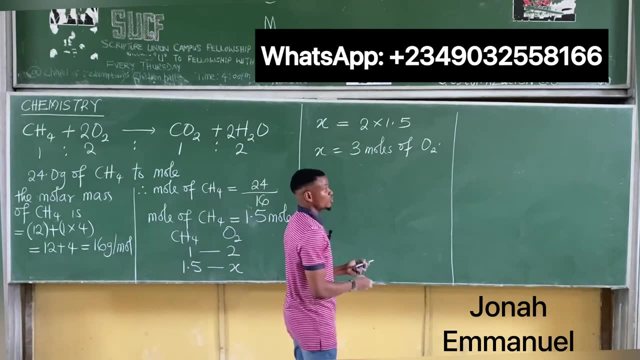 3 moles of oxygen. Please check your question. Will it actually find number of moles or number of mass Mass? So we know to do that right. Convert this to what there Mass. This is mole Check. Your question didn't say if you find the number of moles of oxygen. 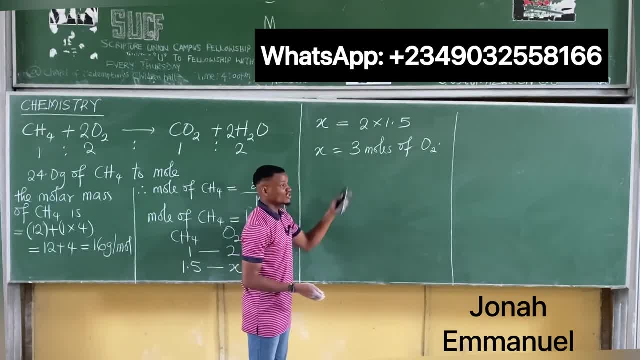 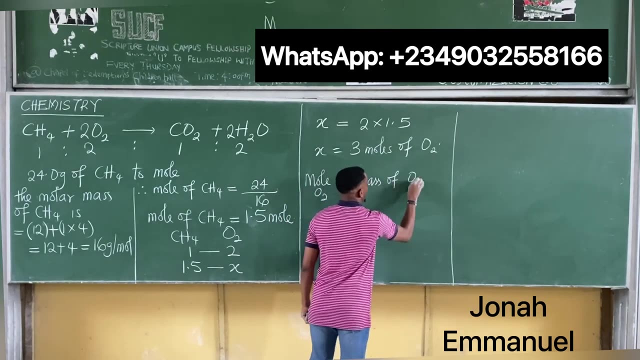 It said mass, Mass of oxygen. I have gotten moles of oxygen. Next up, let me get mass of oxygen. How: We know fully well that mole of oxygen is equal to mass of oxygen all over molar mass of oxygen, Such that if I cross, multiply this and this: 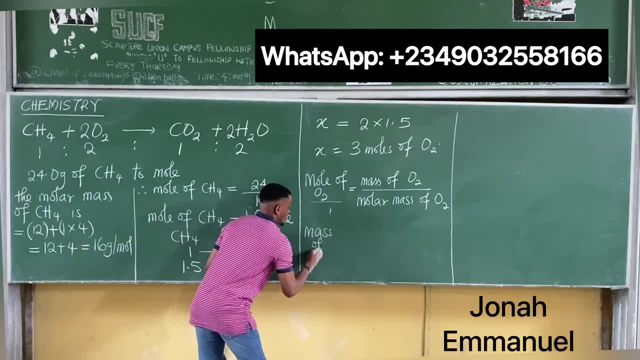 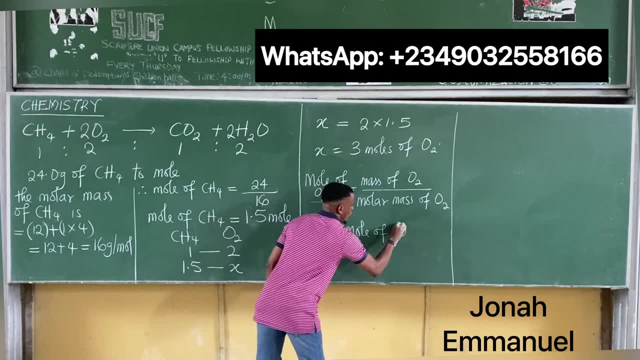 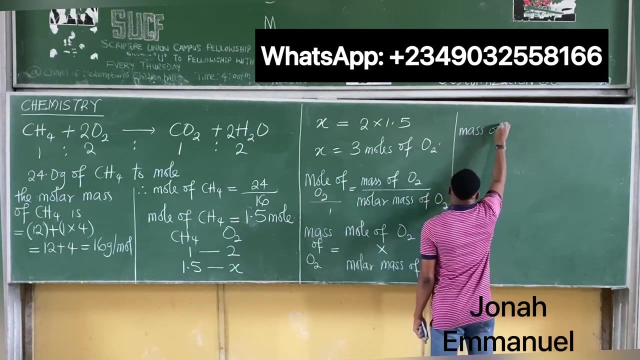 the mass of oxygen. mass of oxygen is equal to this times this mole, mole of oxygen, times this one here, Molar mass of oxygen. So my answer is equal to. that means mass of oxygen is equal to mole of oxygen, does this? 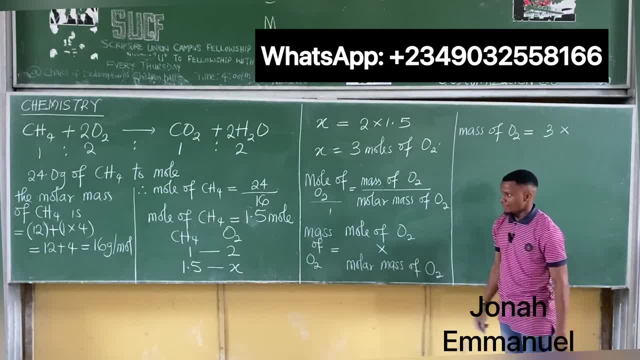 3 times molar mass of oxygen. We have not calculated before, Okay, we have not calculated here, but we know the answer, Abhi, From my previous example. what was the answer? 32.. So please remember how we got. 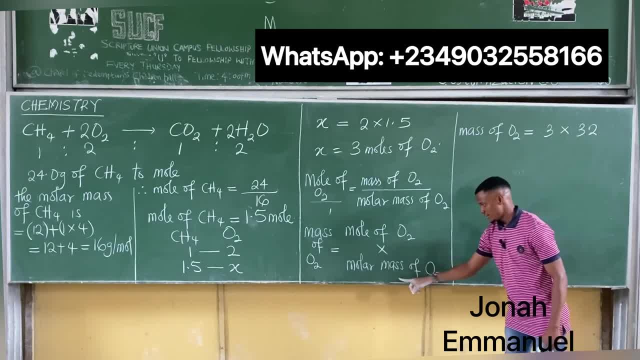 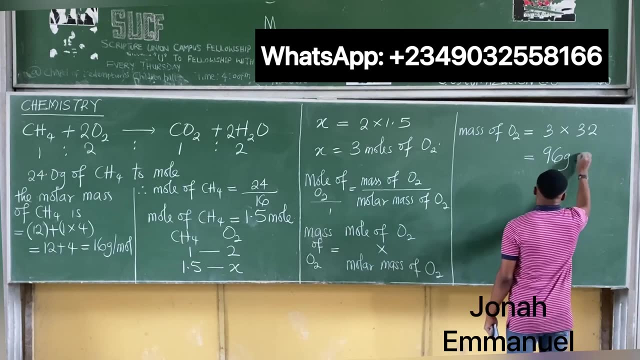 32. Please, please, please, go and check. We calculated this one here For oxygen 32.. Yes, Yes, That was 16 times 2.. Alright, So what's my answer here? 96 grams Abhi Of what there.